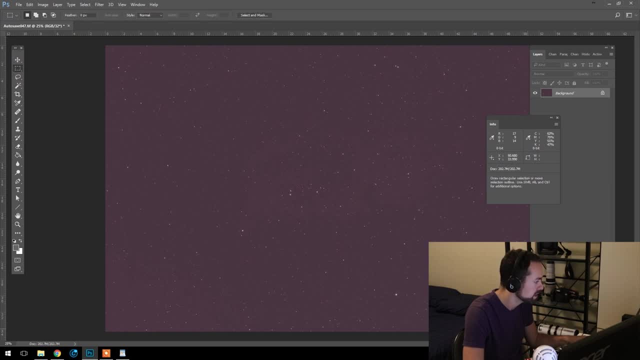 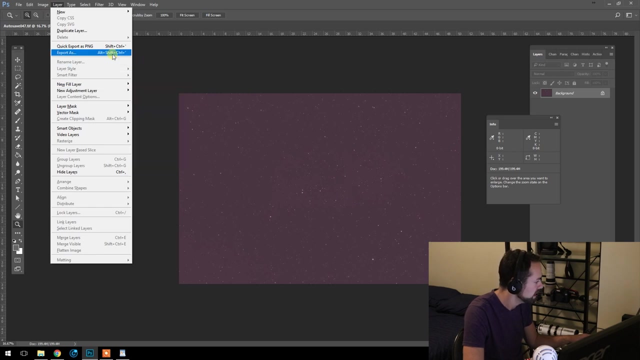 thin line here as well, so I'm gonna crop that out. So the first thing we're gonna do is take a look at the brightest and darkest points of this image. So we're gonna open a threshold adjustment layer. So if you go into layer, new adjustment layer- actually sorry, we have to convert this first. 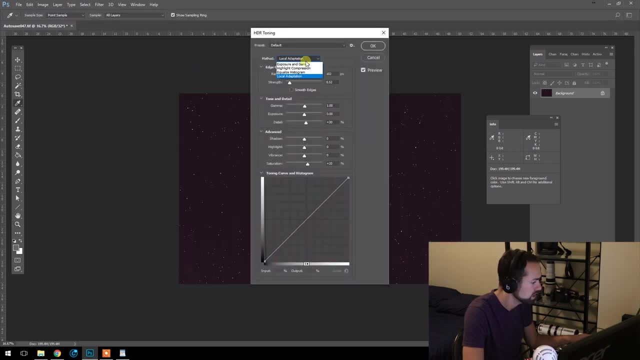 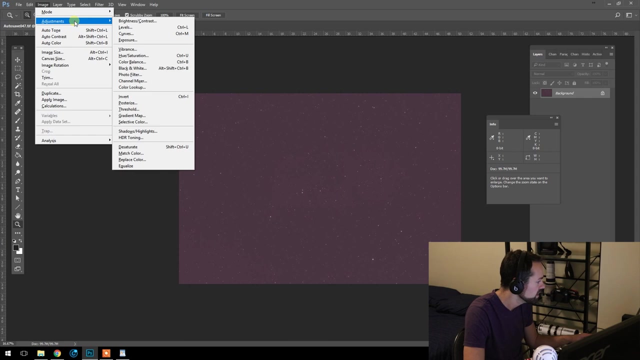 I'm going to convert this to a 16-bit image. The method here is exposure and gamma. Don't use the default local adaptation, So nothing has changed with the image here other than the fact that it is now 16-bit. So we'll go into layers. 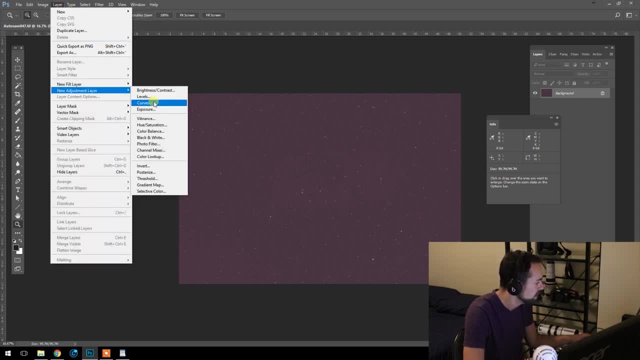 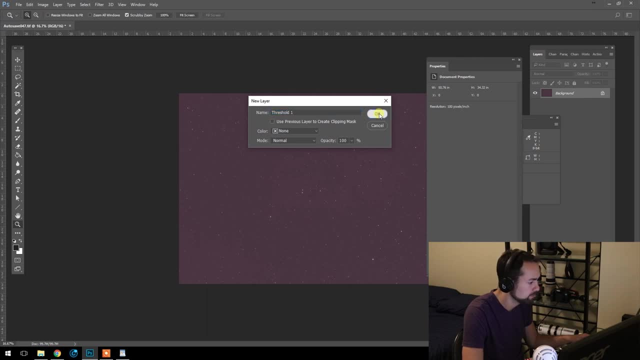 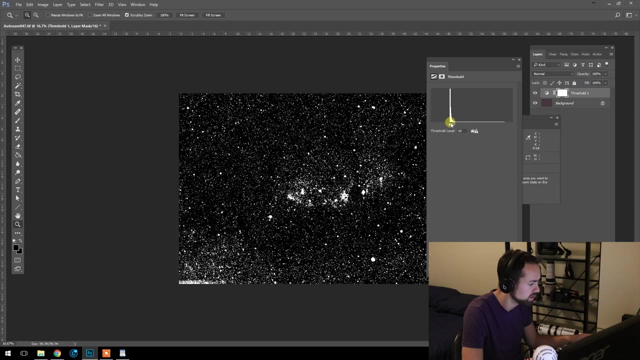 and threshold. Here's the window, here We're gonna say okay, and so we're gonna slide this slider back and forth to see the brightest and darkest parts of the image And, as you can see, as we get around this spot, you can see some of the, the glow down at the bottom left here, the sole nebula of 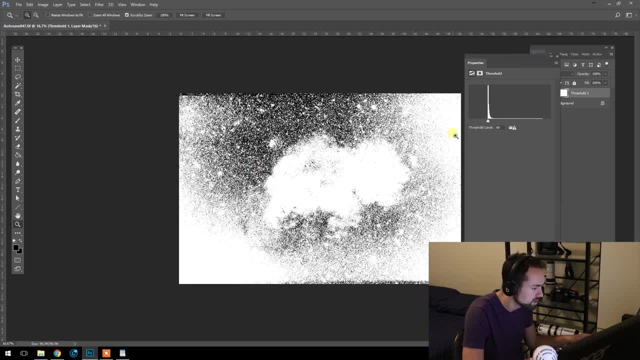 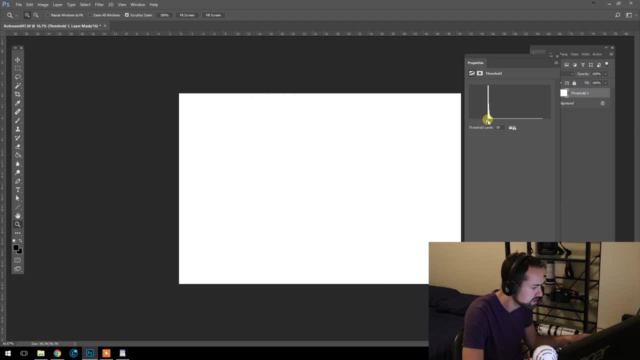 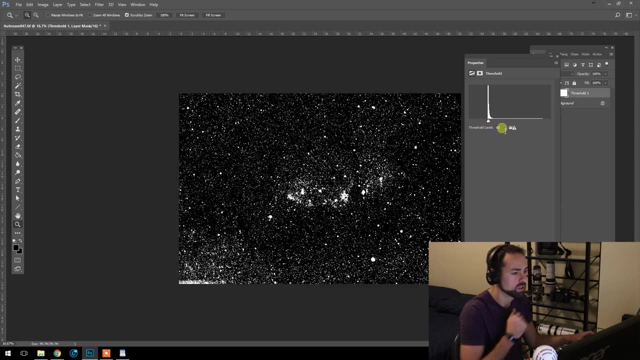 course, and then the darkest areas here. So now that we know that, let's just get it kind of in between here. So it looks like that's about 60- 61.. Yeah, we'll leave it at 61 now and we're gonna place a black sample point on the darkest area. 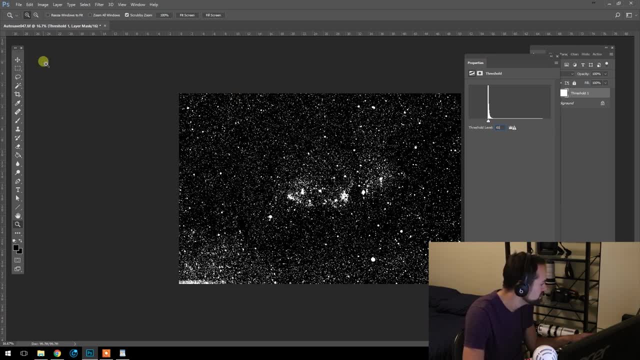 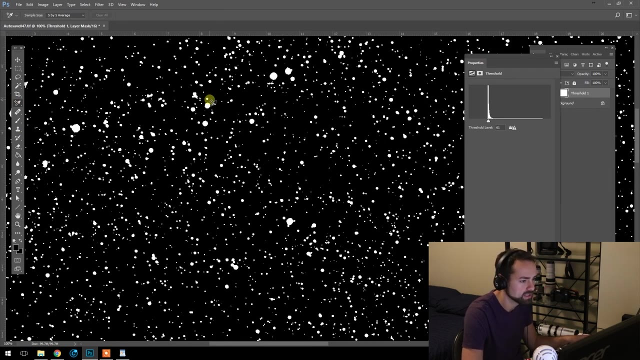 using the color sampler tool here, set to a five-by-five average. And so we know: right here is a dark area of the sky, no stars, no nebulosity. And then we're gonna do the same thing with a ce old media. We'll give it an even value here. 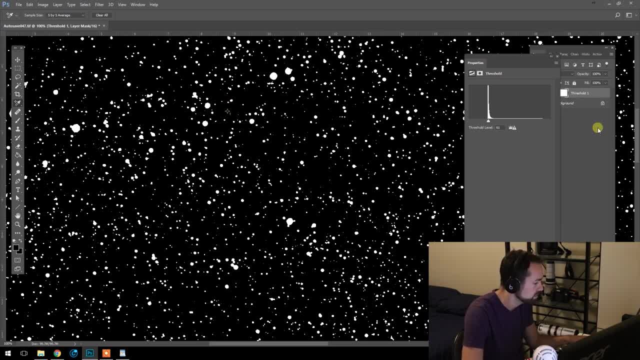 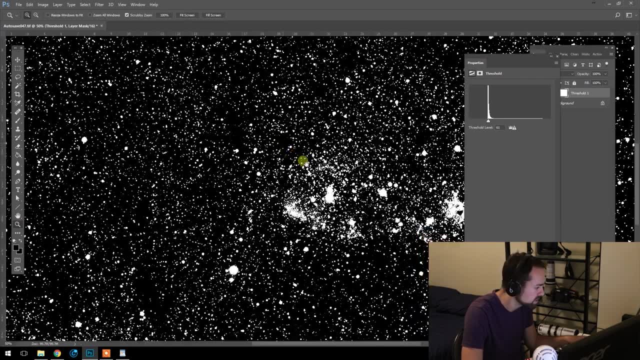 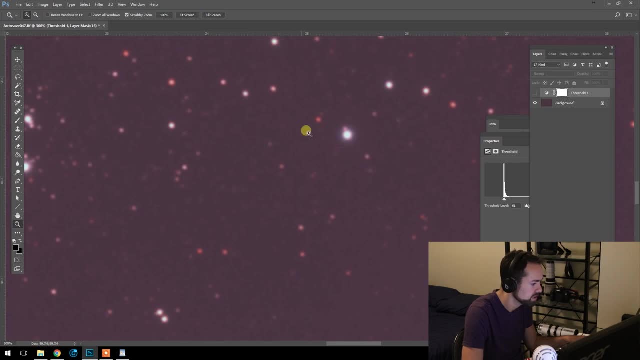 So we're gonna click on that and we're going to 그럼 white the brightest portion of the image. so if we turn this off, we can see some of the brightest stars here, and the cooler, bluer ones are going to be the brightest, so i'm going to choose this one. 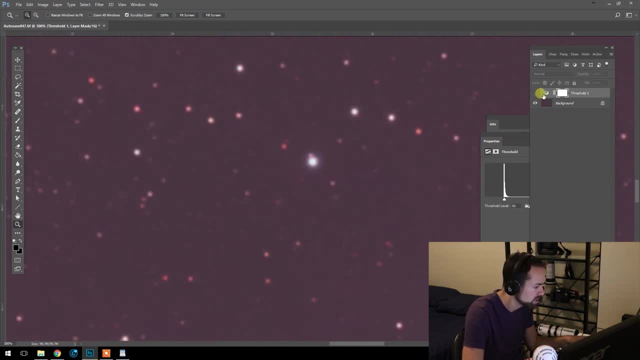 right here and we'll. we'll just turn this threshold layer off and set our white point indicator right here and now. we're going to um turn off the threshold layer. we can just delete it. that was just to see the? uh confirm the darkest and brightest areas of the image, and so now we're. 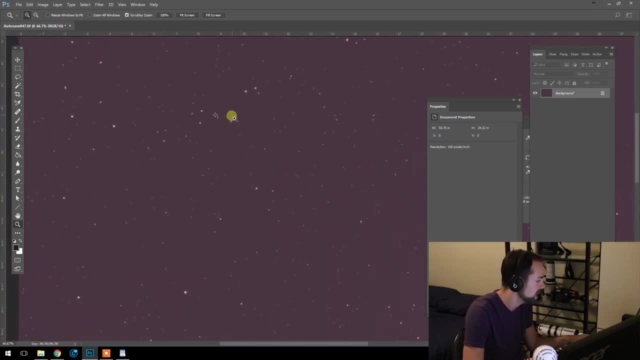 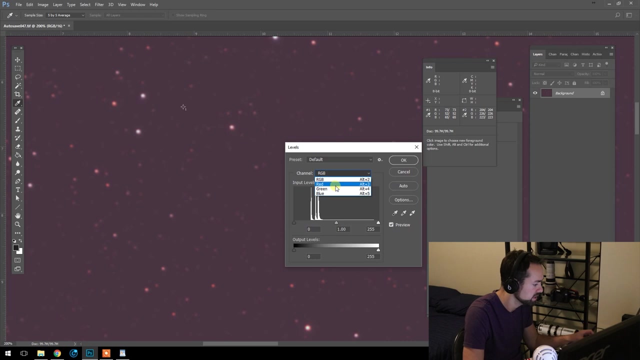 going to control. we're going to adjust the- uh, the background levels, so we've got our point set at one here. so there's the data there, rgb, and those are the numbers, and we're going to move these sliders individually to balance the background. so i'm going to bring this into. let's go 19 across the board. 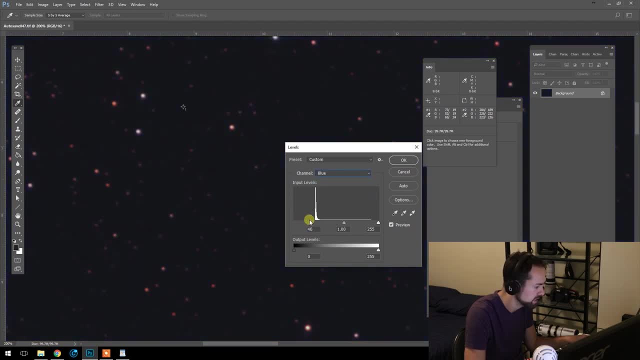 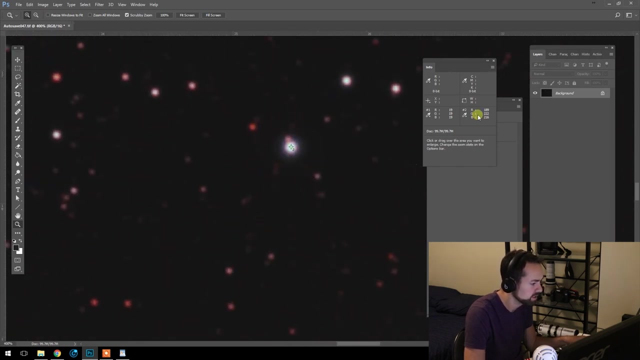 so what we're doing is just setting the black point and getting that balance: neutral, dark background, sky. so, as you can see, rgb levels are 19, 19, 19.. so we've set the black point, now we need to set the white point. so that's indicator 2 here and you can see 189, 222, 216. so the same thing in levels, but this time. 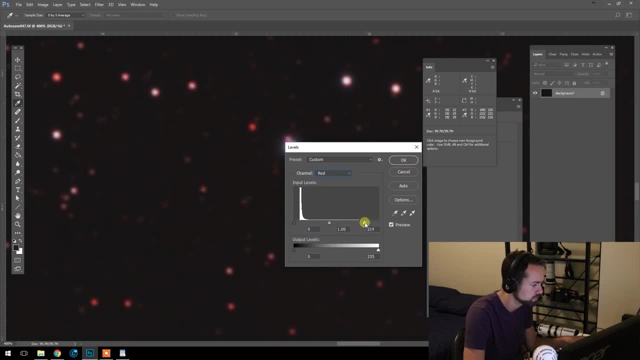 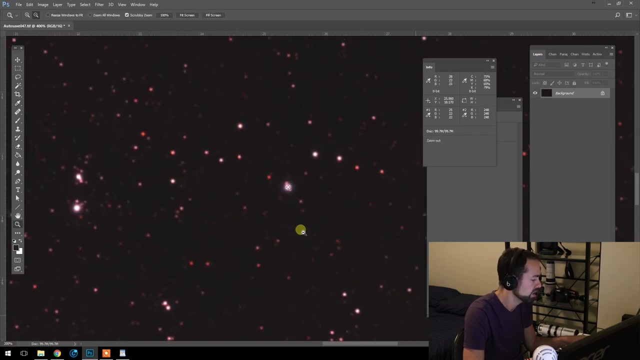 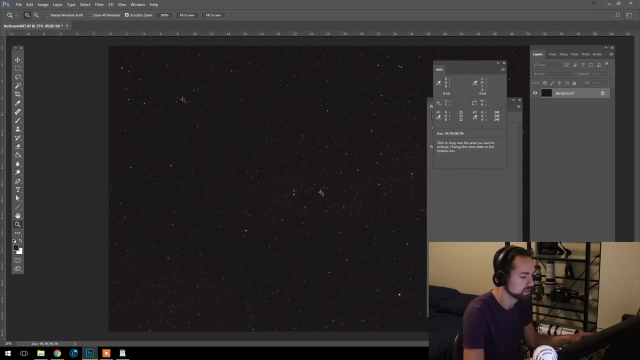 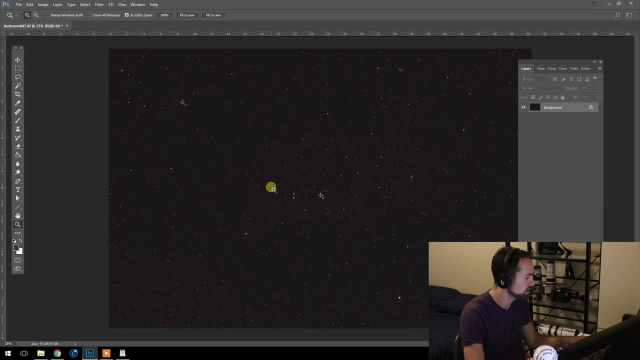 we're going to be adjusting the right hand side of the slider and the number we want is 248.. there we go. now the black and white points have been set in the image. it's a good starting point to start doing some stretching. okay, so we're going to start our curve stretches here and i just want to make 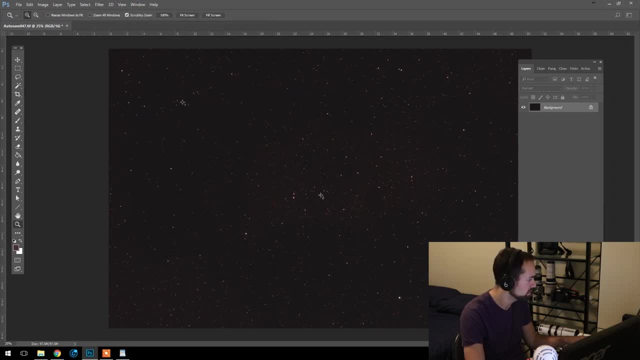 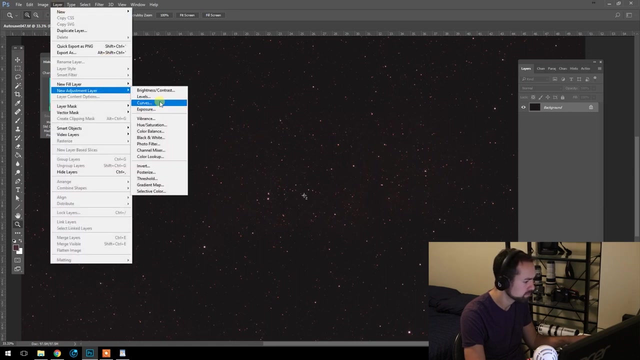 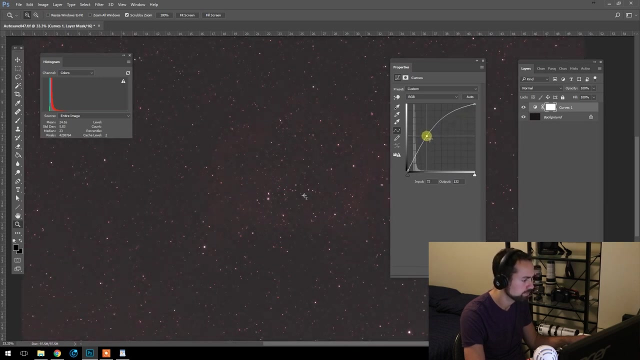 sure the histogram window is open so we can monitor those rgb levels. i'm going to keep it on colors here. so we're going to start a new adjustment layer curves. i'm going to do a modest astro stretch. it's just going to attach this one and this one says: 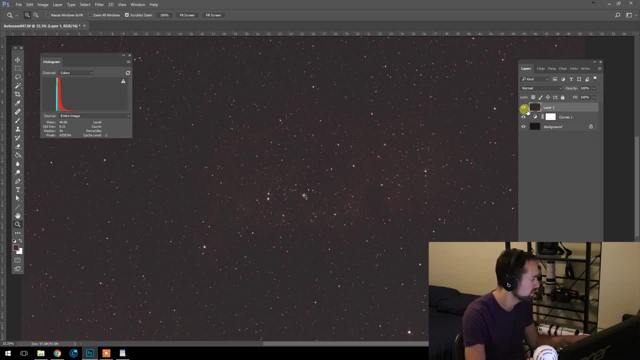 so i'm just going to check my levels. so to do that you can press control, alt, shift, n plus e to do it creates a stamp of everything underneath, all your layers, underneath, and then you have that regular looking histogram. so i'm just going to pull in the 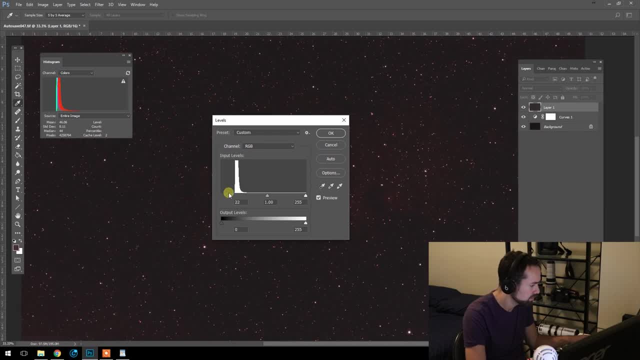 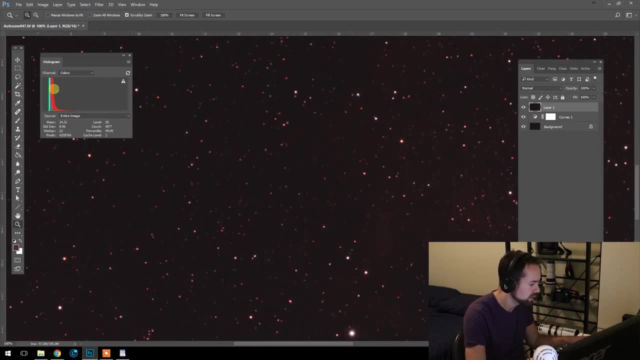 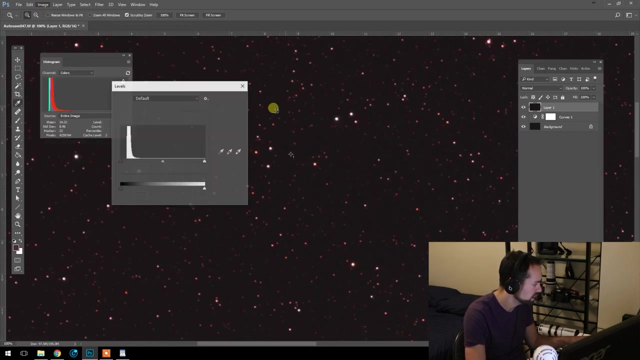 the black point slider here. so i'm just going to pull in the the black point slider here and I can see the red. it's a little overly red right now, so let's just go back to our black point here and check the individual levels. my info palette. 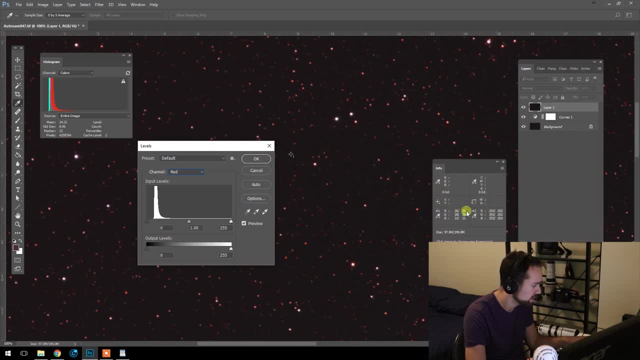 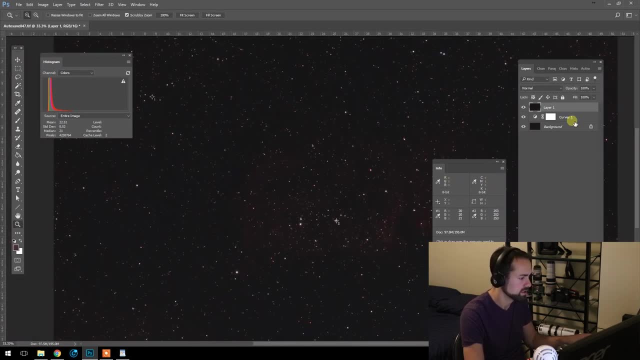 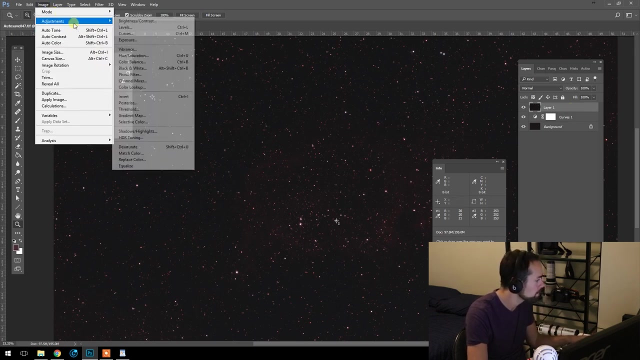 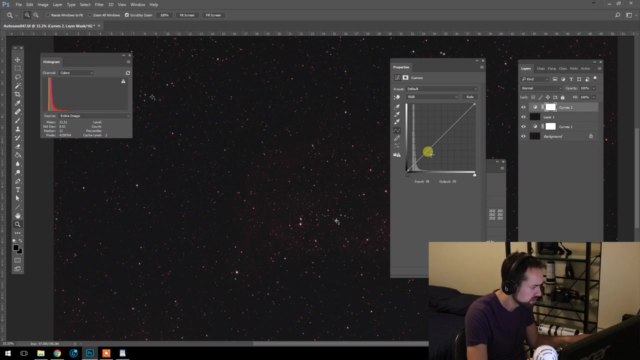 there it is. so, yeah, we're at 26 red. let's bring that back down to 20. okay, we'll do another stretch here, new adjustment layer, and this one's gonna have more of an S curve to it. so I have two points here, and we're just gently pulling that data forward of the nebula, of the sole nebula. 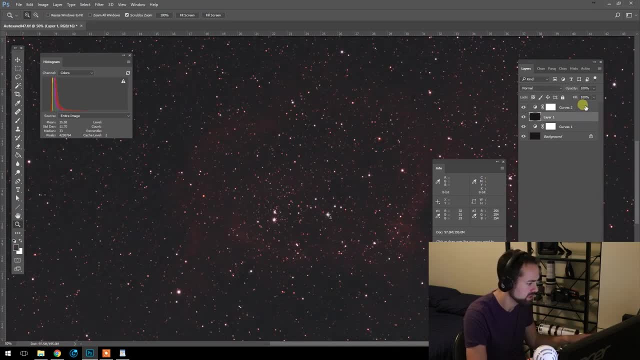 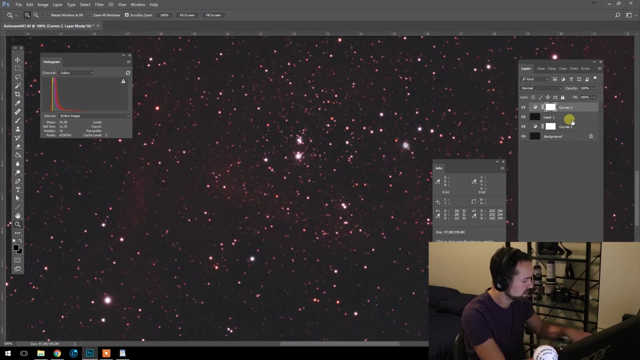 and we're just gently pulling that data forward of the nebula, of the sole nebula. so when you create these new adjustment layers, you can turn them off and on, adjust the opacity and, of course, go back to where you were before the action took place. so again, I'm gonna create another stamp layer on top. check my levels, just. 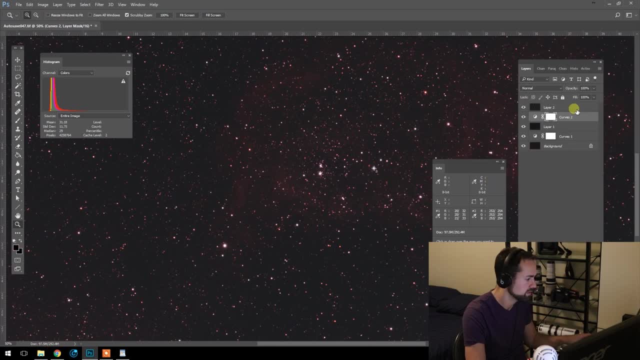 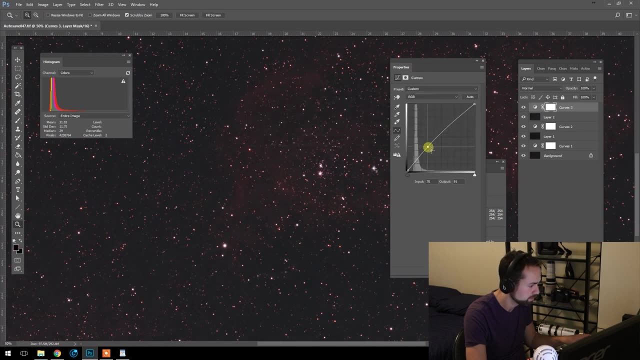 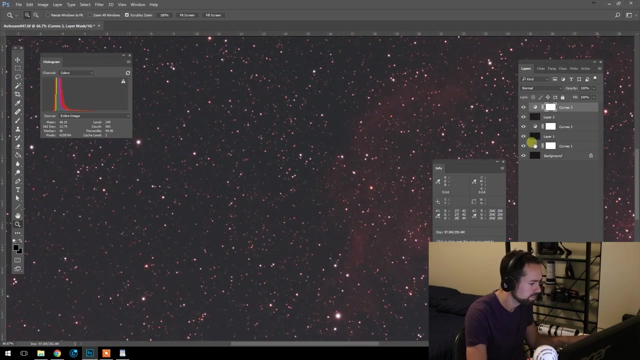 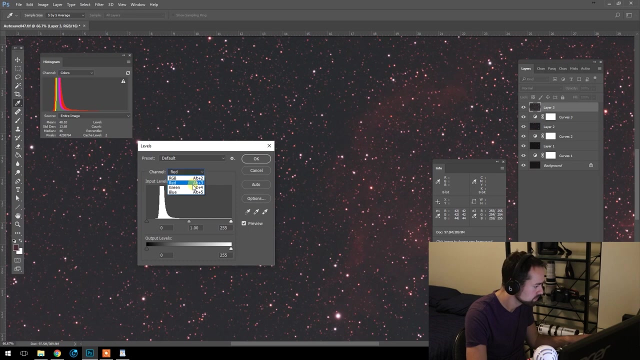 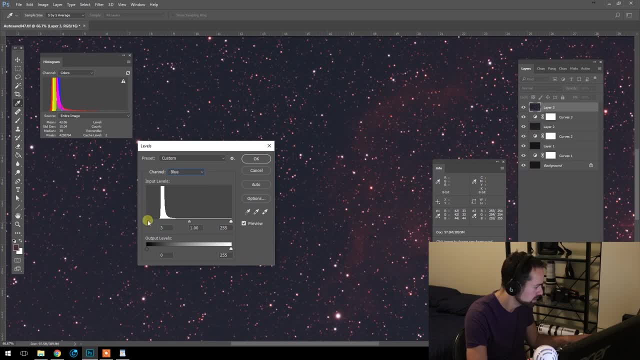 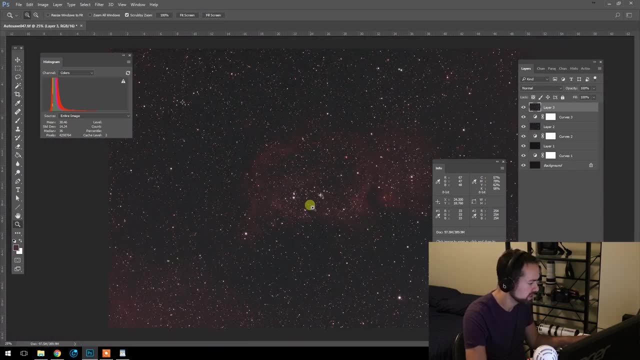 everything to 33, 33, 33, everything to 33, 33, everything to 33, 33. Here we are. so we've stretched the nebulosity, but we've also maintained an accurate color balance, And of course, we can go back and try this again if we're not happy with it. 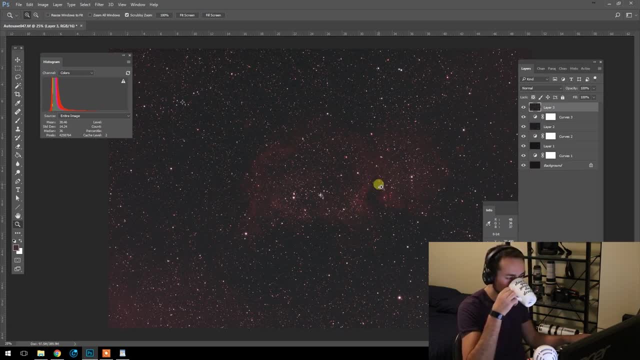 It's known as a non-destructive workflow. But so far so good. I'm happy with this right now. It was a pretty modest stretch, but I don't want to introduce too much noise or bloat those stars any more than I have to. 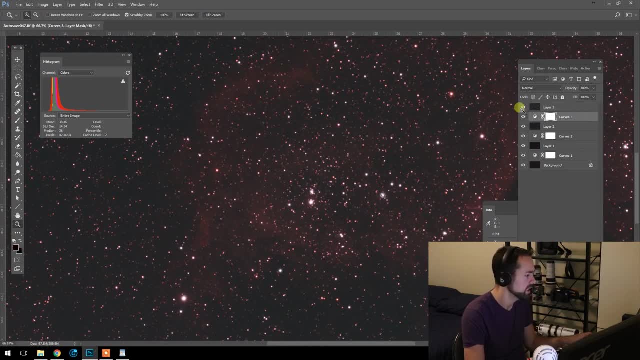 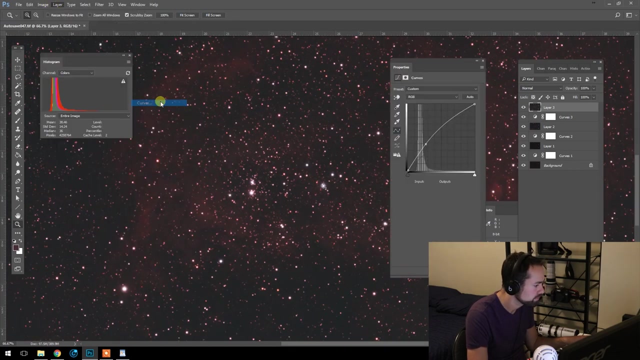 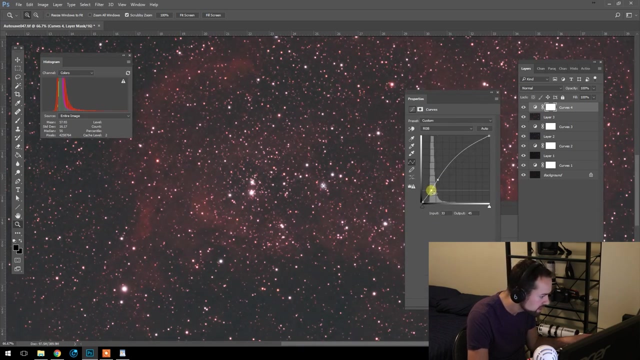 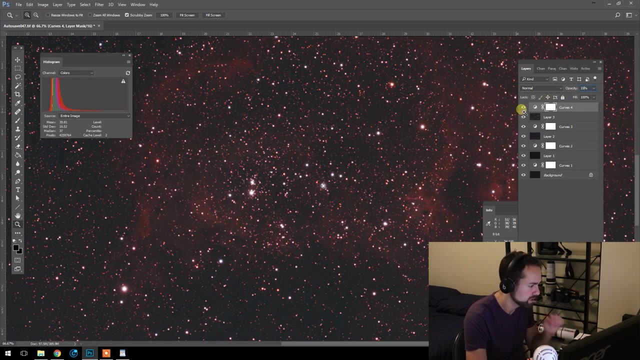 So I'm not very aggressive. That being said, I'm going to do one more stretch because I just can't help myself. What did I do there? Here we go. I closed it. Just an S curve here, And this one. I'll just adjust the opacity layer to about 33%. 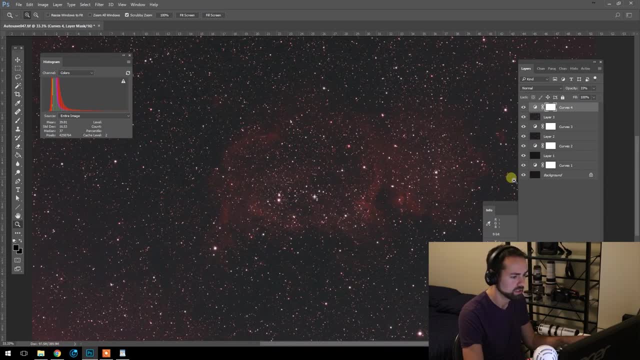 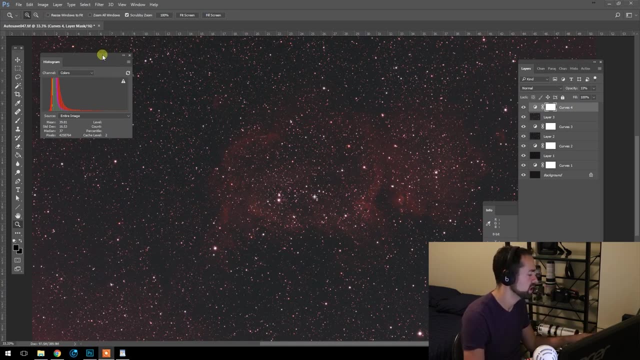 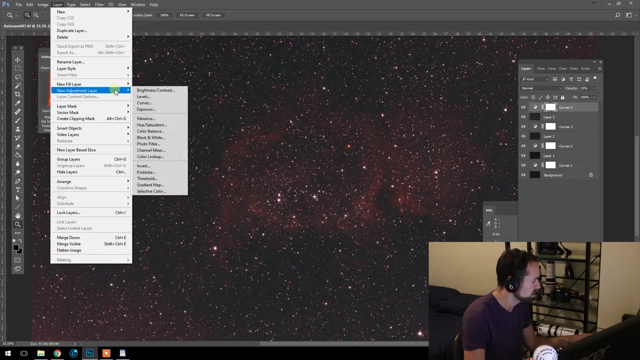 Just a subtle change, a little extra glow there. So that's our curve, Curve stretching. I'm just going to try one additional color correction trick at this stage, By opening a new adjustment layer Curves, this time setting the blending mode to Color. 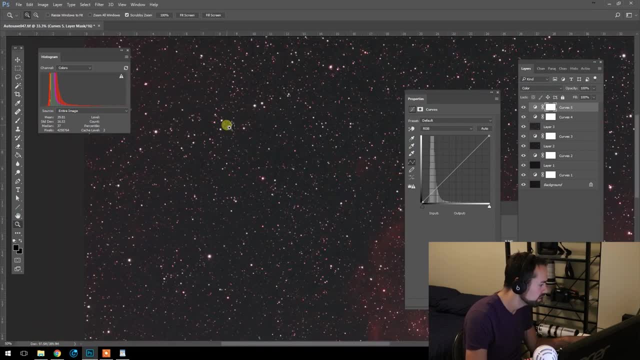 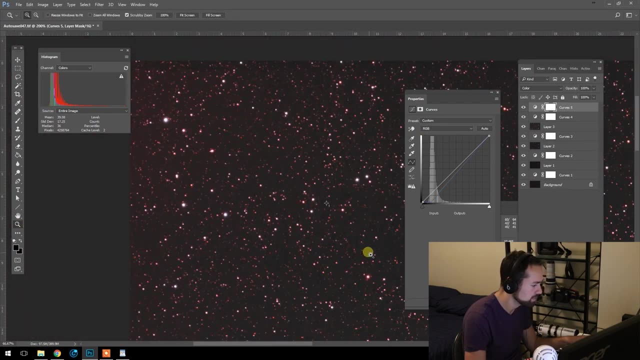 Using the black eyedropper here Choosing a dark area of the sky. So let's set the black point. I like to be a little bit more subtle, I like to be a little zoomed out actually for when I do click this black point, because 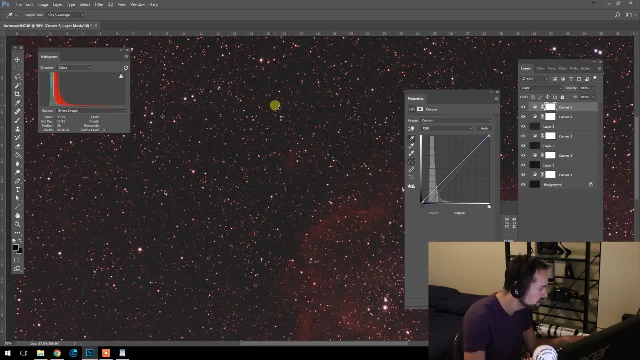 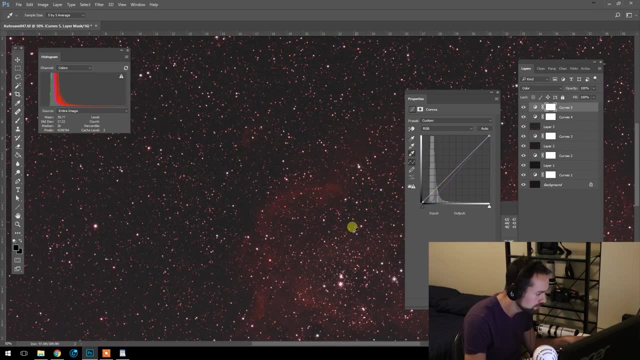 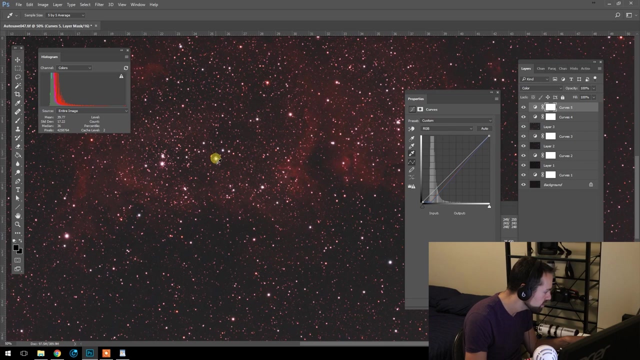 you kind of see the image as a whole as opposed to that isolated area. There we go. I like my images a little cooler. And then now I've just clicked the white set white point eyedropper here And I'm going to click right into our what I hope is a G2V star like our sun. 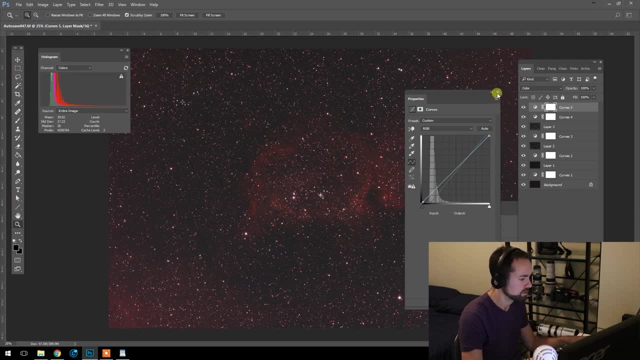 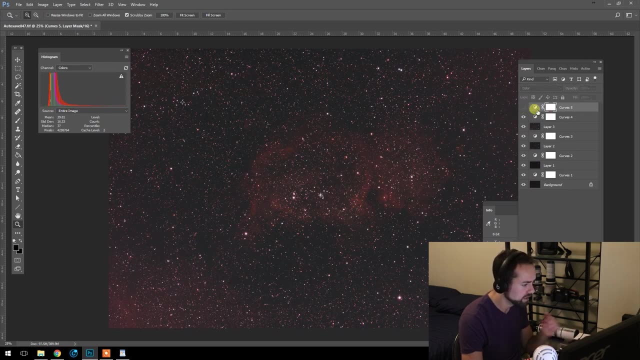 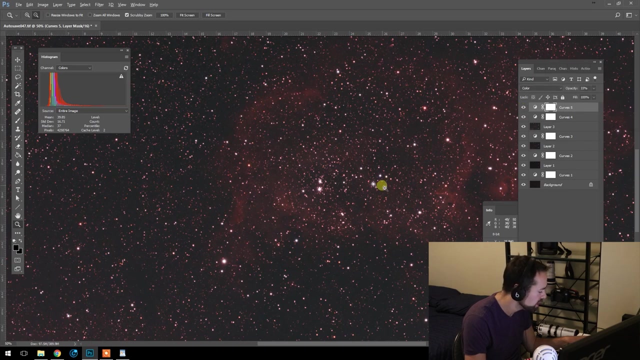 Let's just take a look at that layer. I feel like things got a little too red there. I'm going to bump this layer down When in doubt whether it helped or not. set it to 33% opacity. Subtle difference. 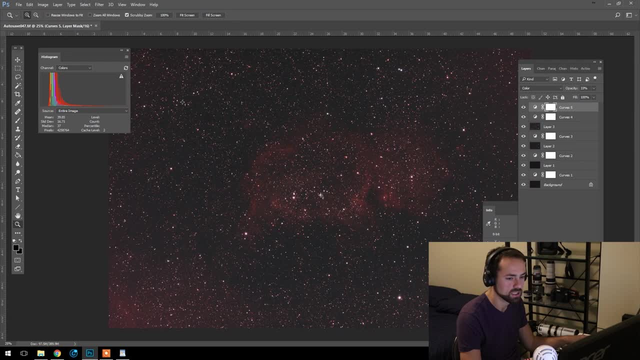 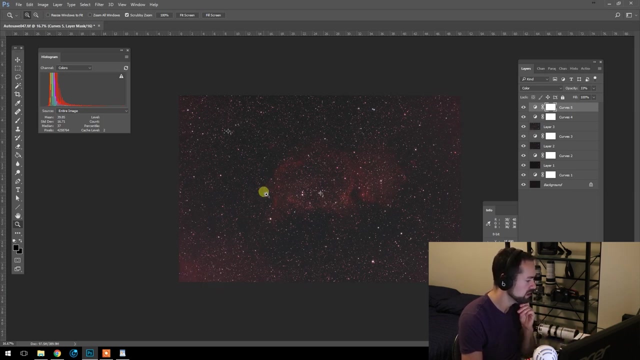 Best of both worlds. So that was just an additional color balancing trick you can try out. So at this stage we're going to remove the gradients in the image, And the fact that there's the glowing portion of the heart nebula down there makes it a. 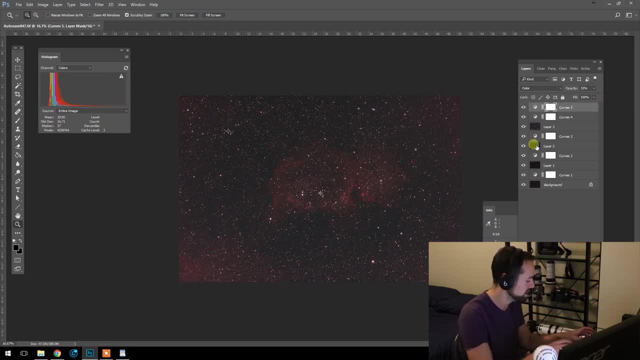 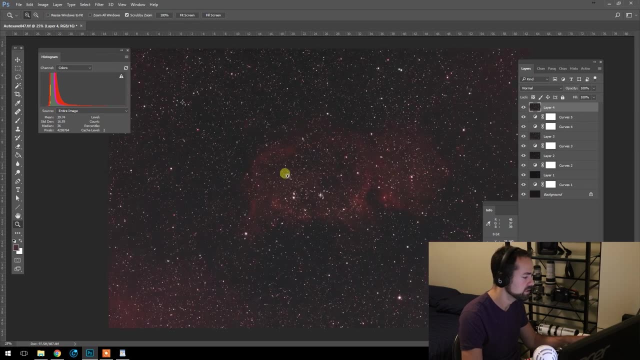 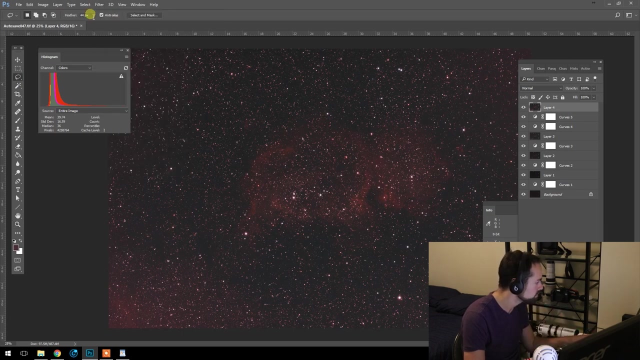 little tougher, but it's not to say that it can't be done. So I just hit control alt and shift control alt And that's it. I'm going to hit control alt and plus E to create my top layer here, And this layer is going to be our gradients adjustment layer. 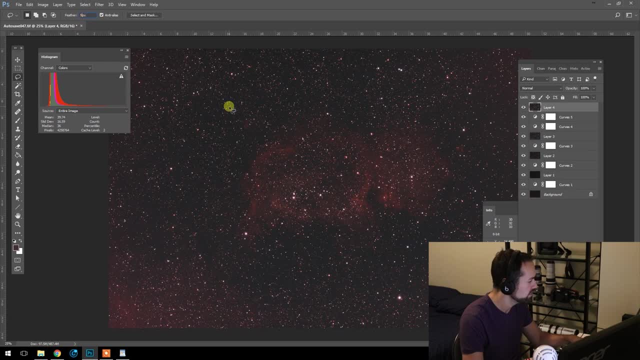 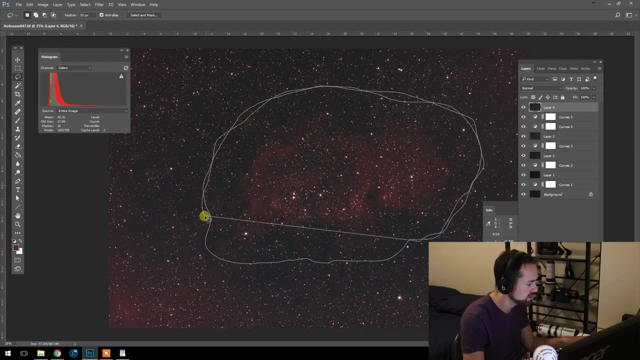 So I'm just going to choose the lasso tool with a very high feather on there. I've got 55.. I don't want to touch this area of the photo And I'm going to save the heart nebula slightly And then select the inverse. 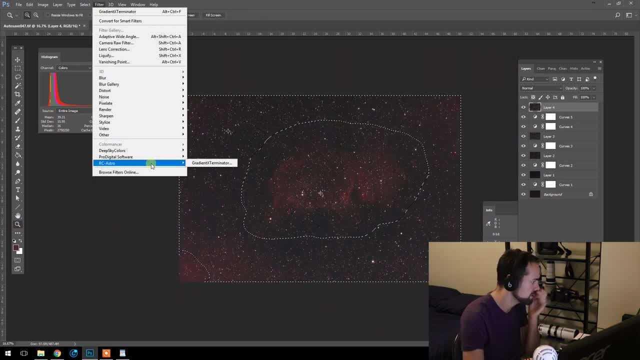 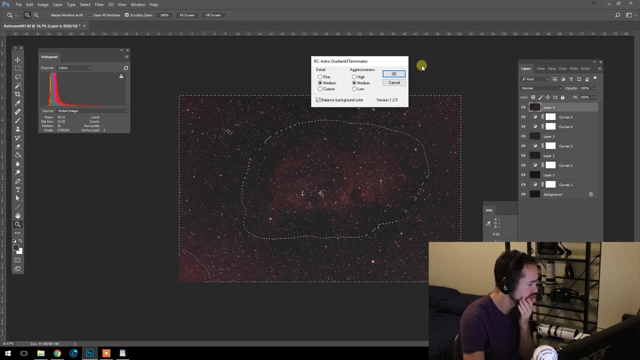 And this is what I'd like. This is the area I'd like to balance. I'm going to use RC Astro gradient exterminator and this is a plug in that I purchased- I think it was about $50, but I use it for every image, so it was well worth it. 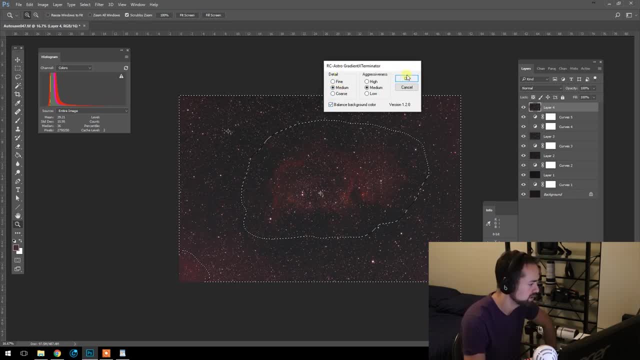 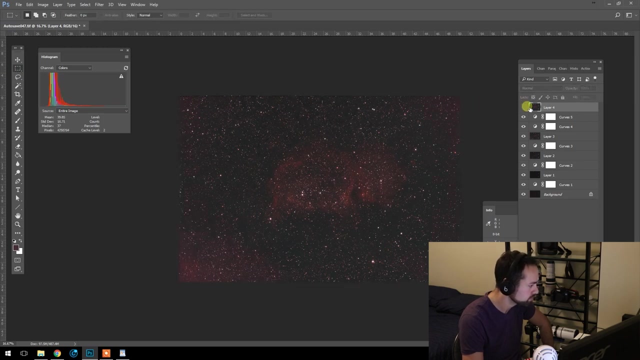 I've got the details set to medium and the aggressiveness set to medium and balance background color checked off And we'll let gradient exterminator do its thing. Yeah, There you have it. So it did fix a lot of the. the gradients were having the glow at the edges. 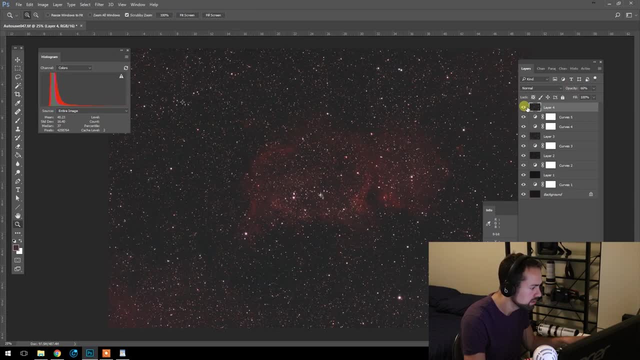 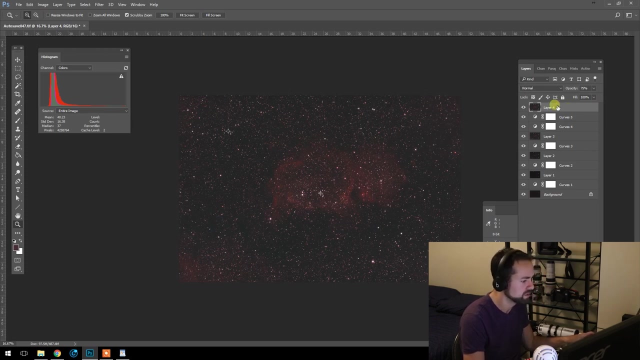 Still gonna play with the opacity a little bit. Kept the heart nebula in there, So I think we'll keep that. You can run this several times if you want. I Think I'm gonna keep it, but about 75%. Any tweaking we'll have to do later is fine with me. 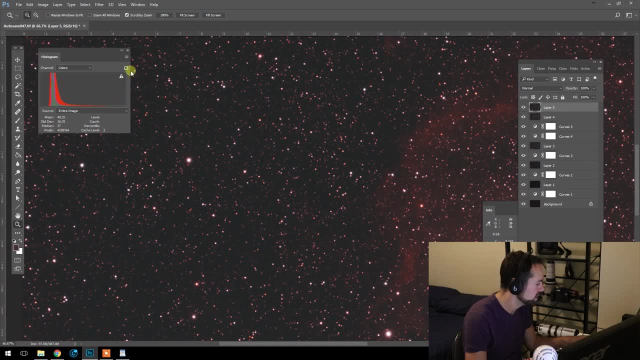 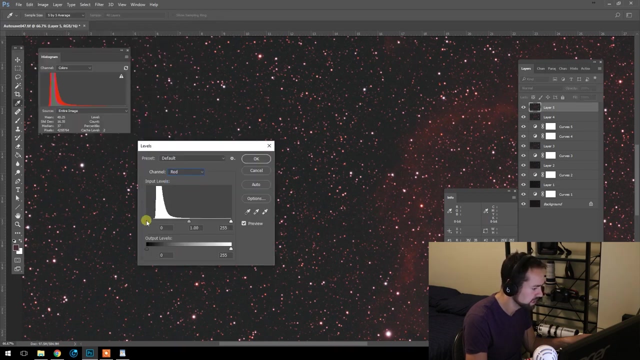 Create a new layer and just check on our levels again, always checking the histogram, checking our color balance along the way. So I can see our black point is here: 35, 36, 34, I'm just gonna balance that out. If anything, I like the blue, the blue channel, to be a little bit stronger than the rest. 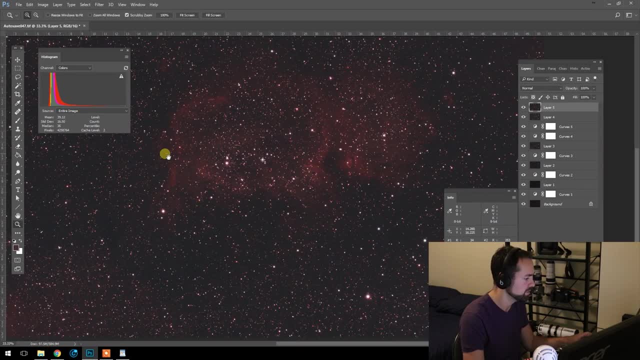 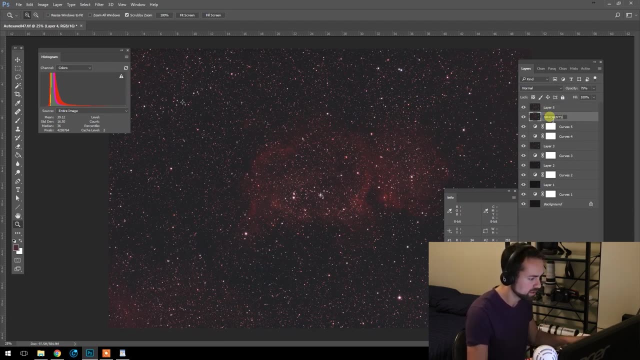 There we go. That's a better color balance. I like what I'm seeing at this point. So if we wanted to stay really organized, we can name that layer gradients And this one color balance. Obviously, if you have more time and you're not shooting a tutorial YouTube video, you can really take your time. 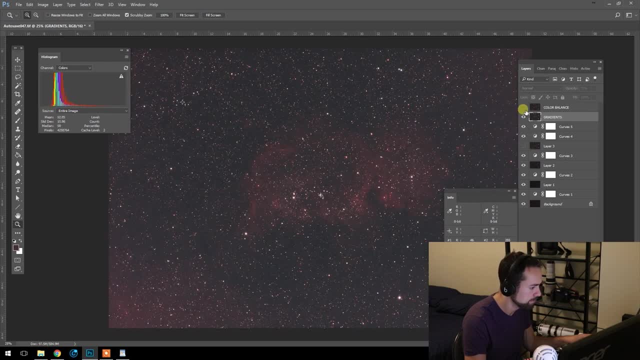 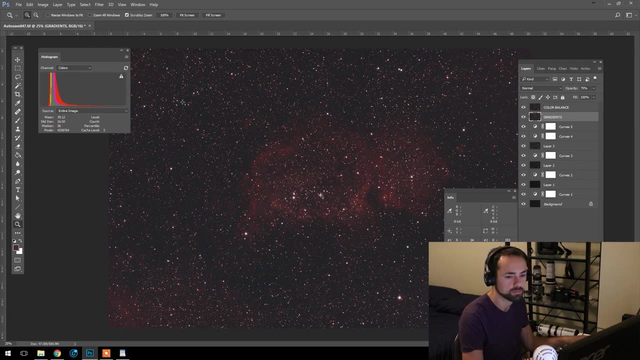 Go back, turn these layers off, try something new, But for the purposes of this video, I think you get the idea, so let's move forward. So this would be a good Point: to save the image as it is or earlier along the way you can save before doing each stage. 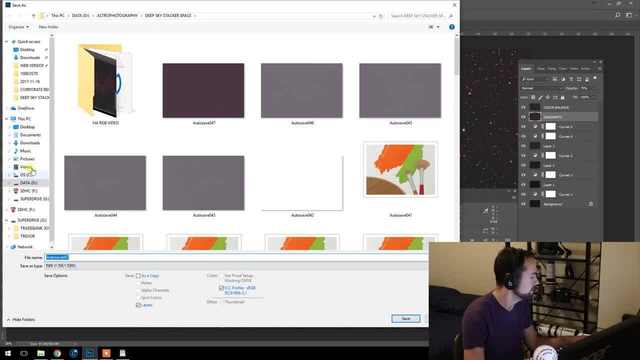 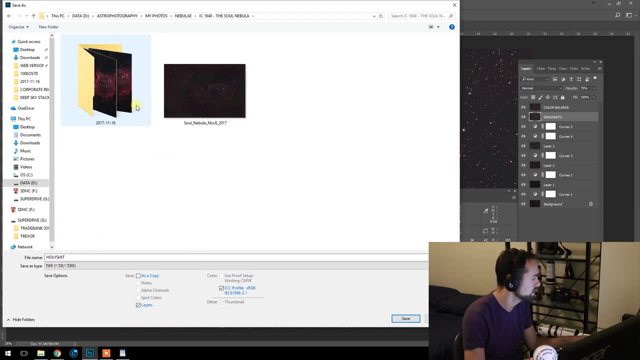 Just so it's easier to get back to where you were. I'm gonna save this. I save my folders by month and date. today is the 17th. Ignore that file name: soul 2017- 11- 17. Then I say this, with the layers: of course it'll be a pretty big file, but be nice to go back here. 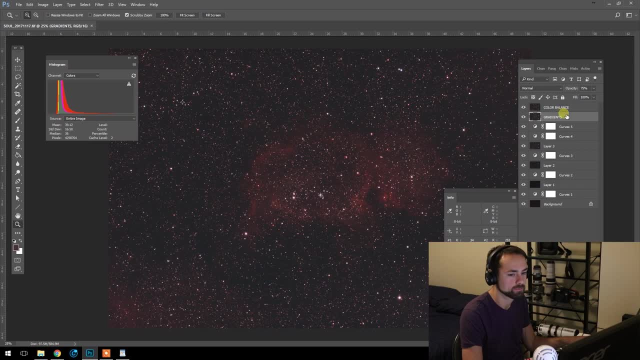 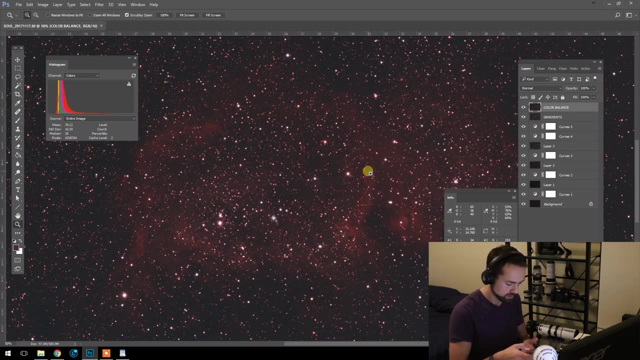 You know you're going to have to redo those things And then you'll have to color your ones And try to make sure you get the kinds of colors that are available. So we'll just go go back and out of your software and make sure you're able to see your assets. 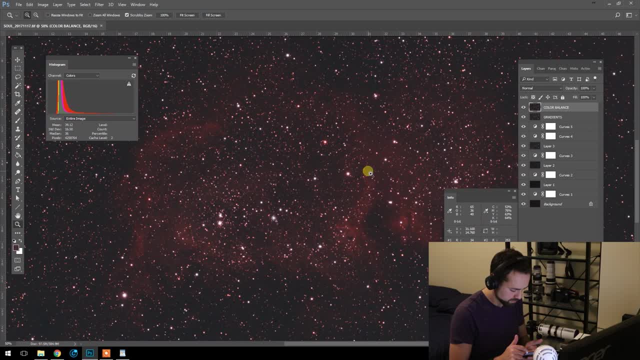 And then you can do the actual color saturation. Okay, so let's do this. Okay, now we're going to do a color saturation. Okay, now we're going to do a color saturation. Okay, so now we're going to do some color saturation, increasing to the nebula itself. 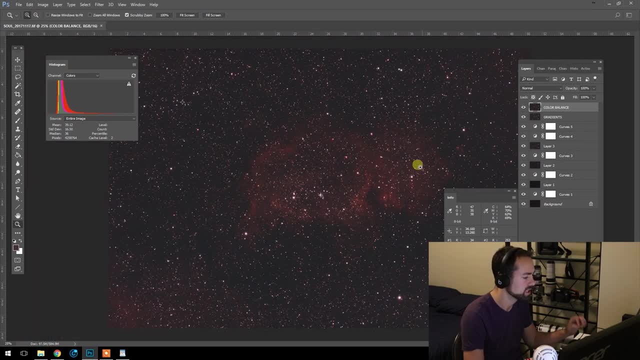 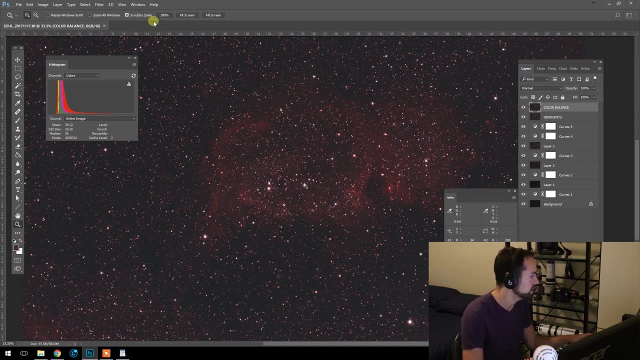 of course. so we'll need to isolate the portions of the image we want to boost in color and the ones that we don't. So a great way to do that is with the. so we'll start a new layer here. Actually, we'll wait until we make our selection. 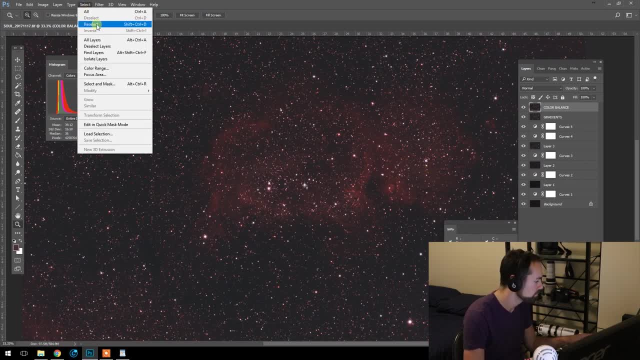 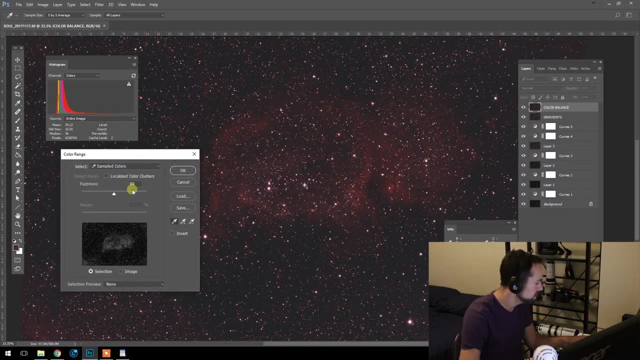 So select color range. this is a very powerful tool for masking stars and the nebula. So we have it set to sampled colors here and I'm going to pick the use the eyedropper and use the pink. So we're going to pick the eyedropper here. 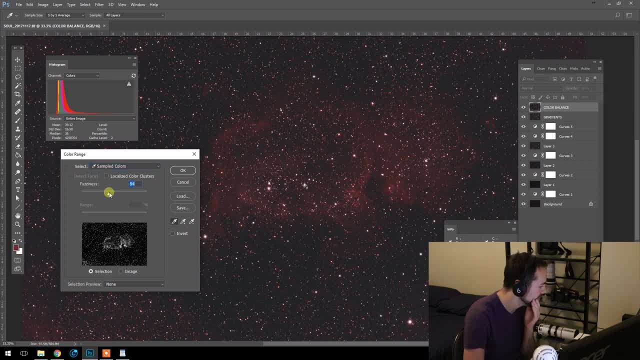 I'm going to pick the black one, I'm going to pick the blue one, I'm going to pick the purple one, And then we're going to do a little bit of color saturation, a little bit of color saturation here, And then we're going to do a little bit of color saturation in the nebula here. 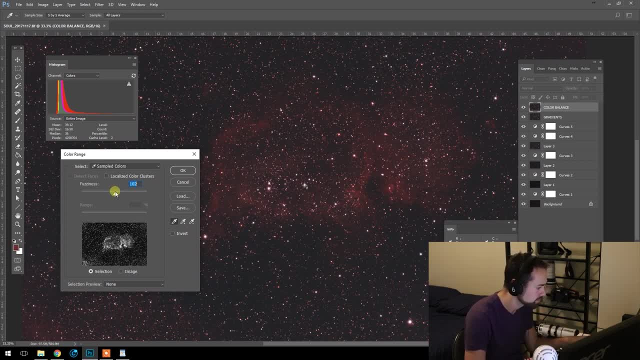 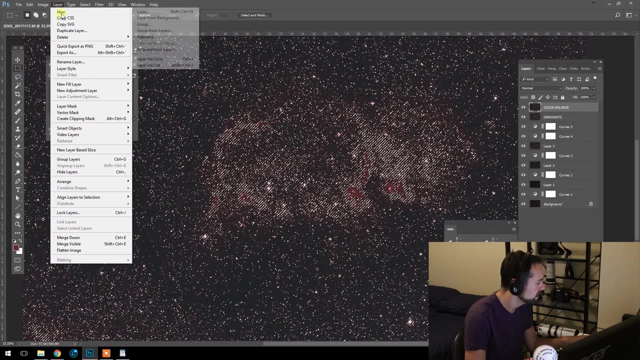 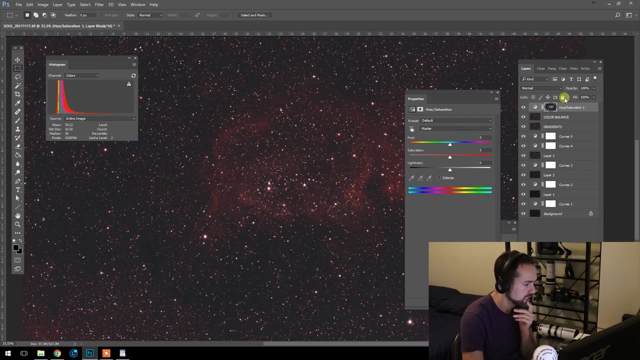 And then by adjusting this fuzziness slider you can isolate a pretty well, just the nebula here. And so now that it's created that selection, we can do a new adjustment layer here- Hue saturation, and lo and behold, it's created a mask from that selection. uh, for us to. 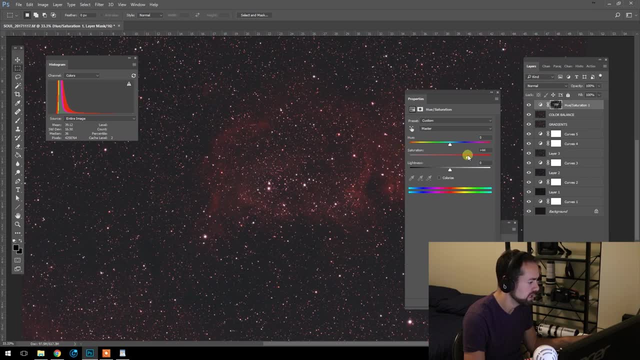 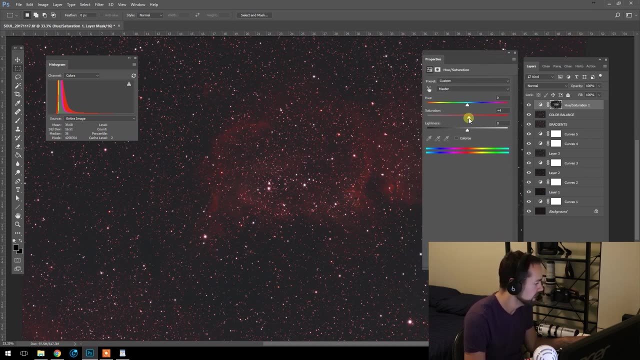 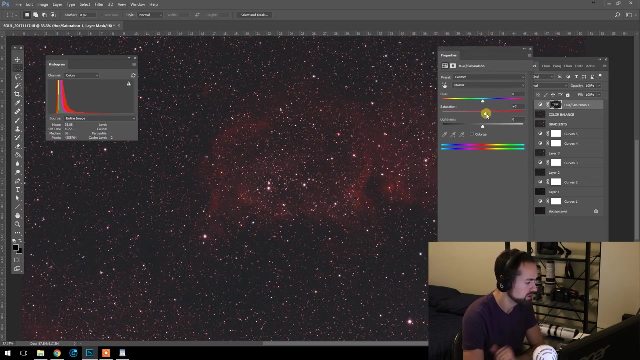 adjust the saturation independently from everything else. Uh, Pretty cool. Uh, this is really where your personal tastes come into play. Um, I think I'm somewhere in the middle. I don't like the super vibrant- uh, really rich color images, but I don't like the dull. 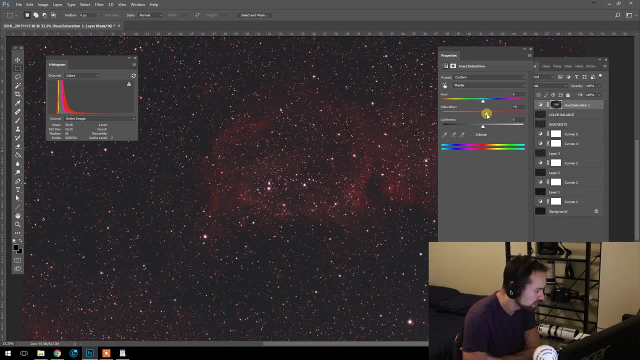 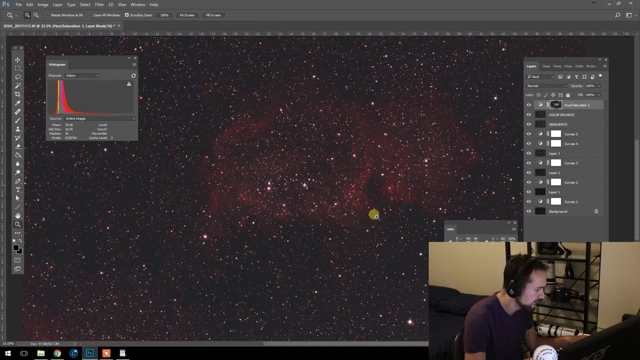 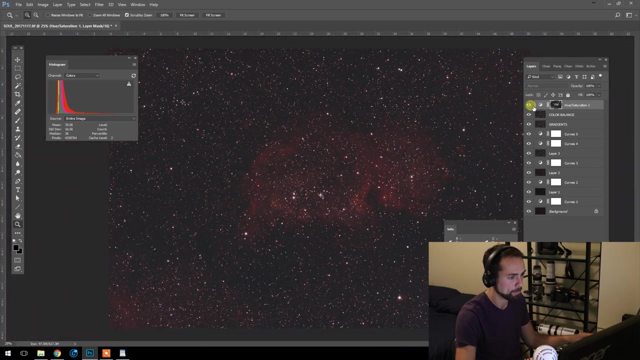 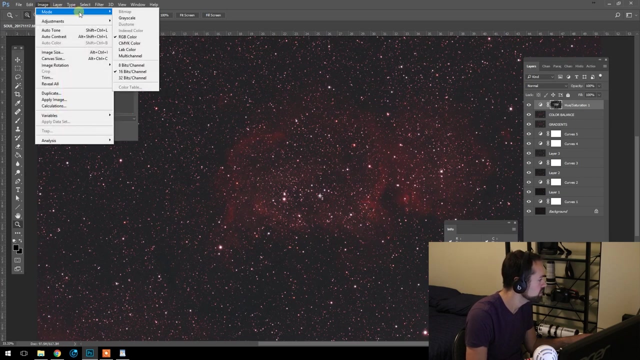 ones either. Um, I am going to go saturation boost of about nine and let's turn that off and on. Okay, Cool. So here's before and after. So pretty subtle, pretty subtle change there. You can do the same thing with the. uh, I like to do the vibrance control. 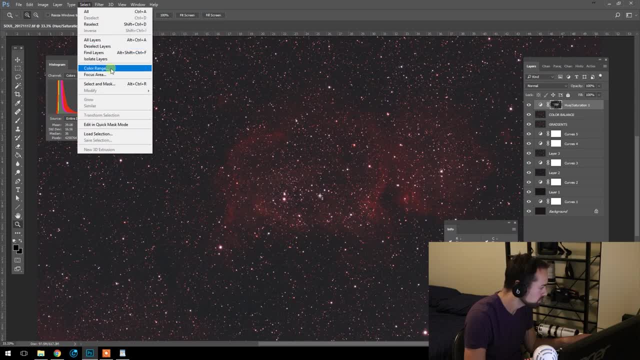 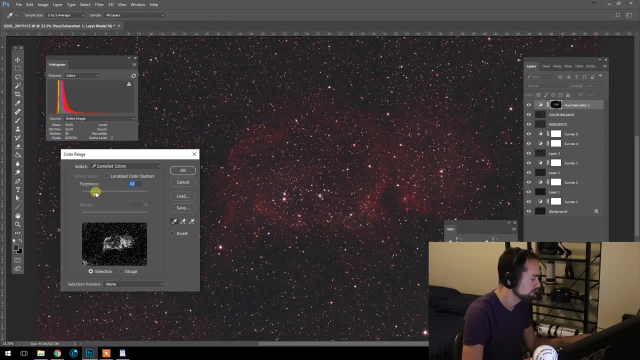 So we're going to do select color range again. Okay, Cool, Sampled colors. I'm on my adjustment layer by accident. Color range, Sampled colors. All right, I just want to make sure that I'm in the right place. 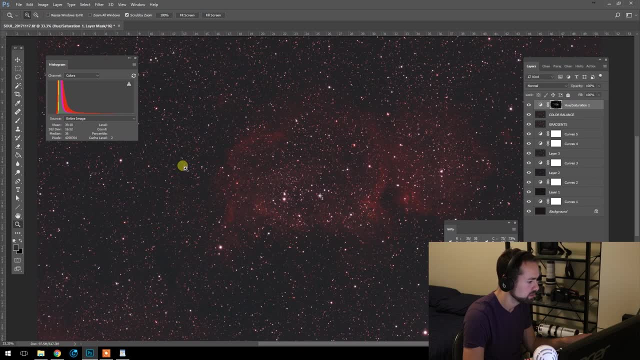 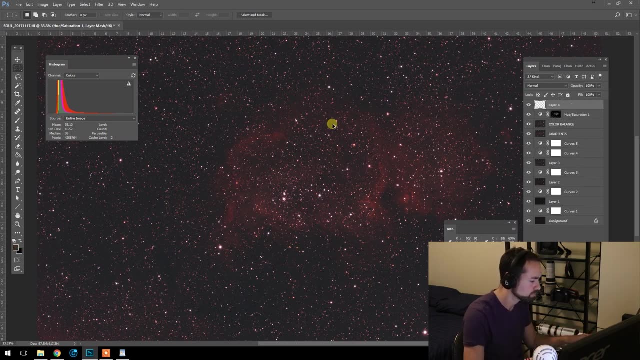 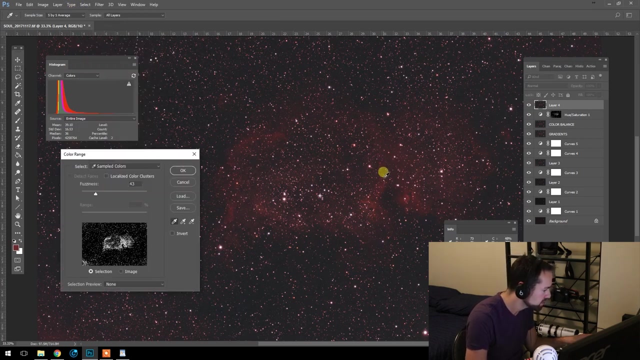 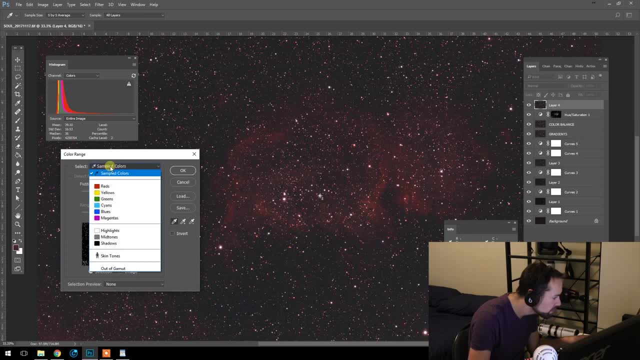 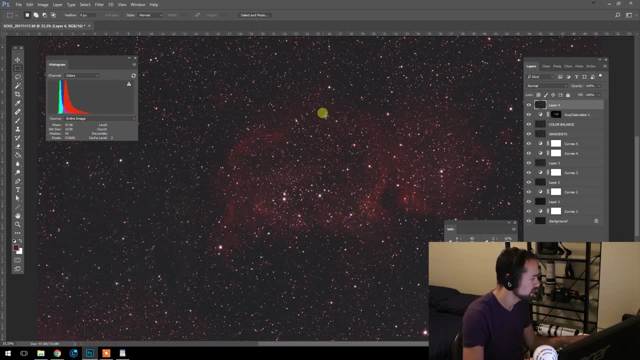 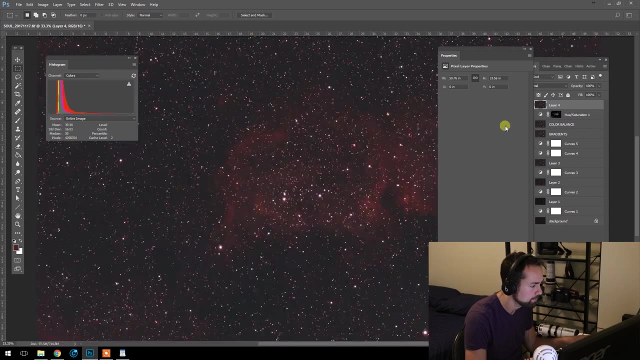 Cool, Cool, Cool, Cool, Cool. Okay, You just want to make sure I'm on that Pink, Okay, Okay. Okay, Selection is made. layer vibrance this time. Boost the saturation a little bit and the vibrance. 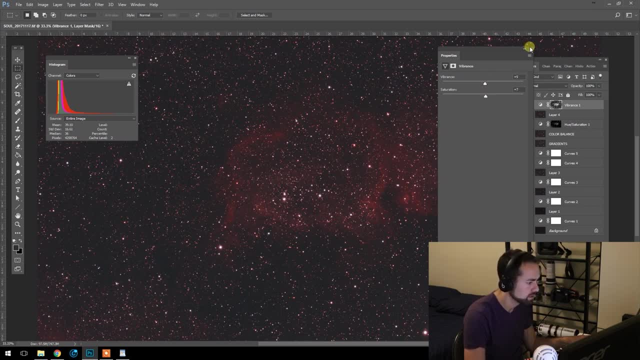 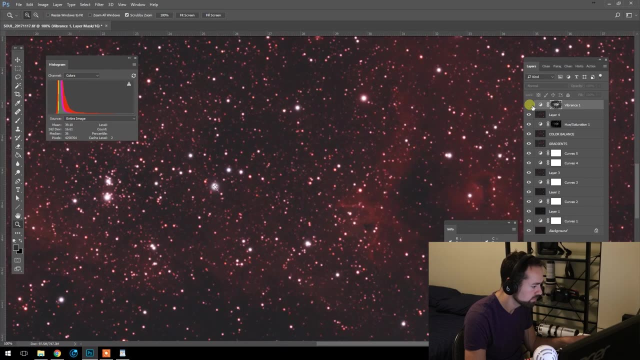 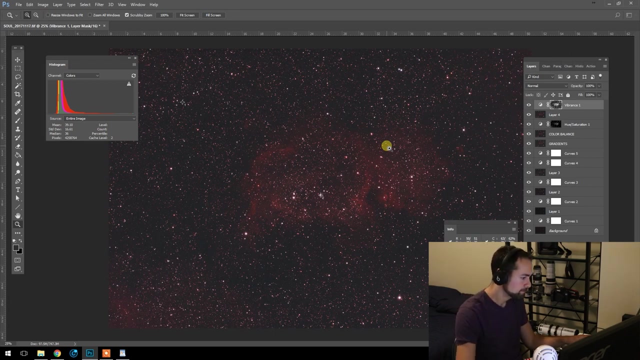 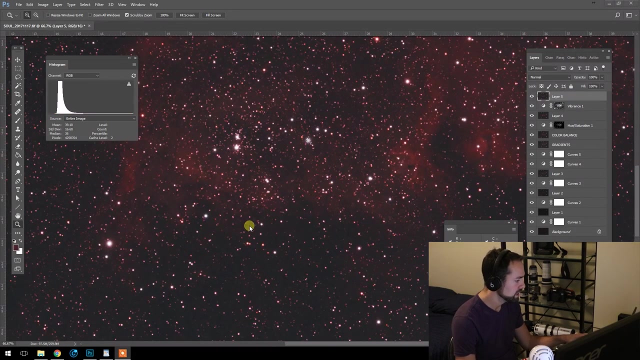 a little bit, Okay. Okay, the before and after We've boosted the colour. Next we'll move on to noise reduction. Okay, so, to speed things up, and since I won't be going back in this tutorial anyway to any of the previous stages, I'm just going to merge these layers just to speed up my. 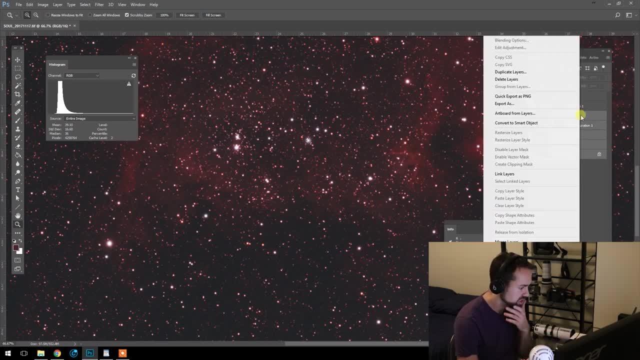 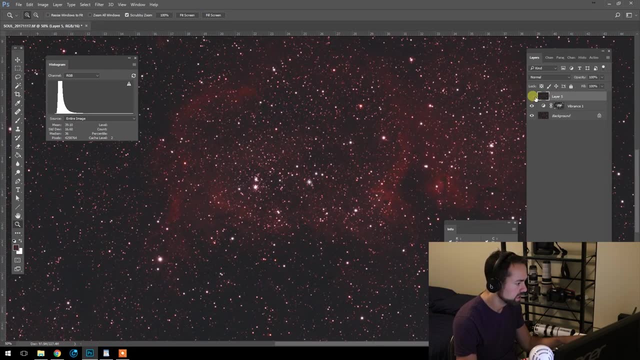 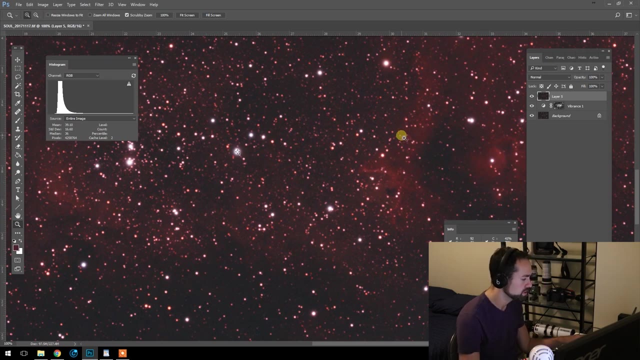 machine, Everything actually underneath our latest changes. I'm just going to merge. Okay, so I've got another layer on top here that we're going to do our noise reduction on. So this is the first time we're going to be using the Astronomy Tools action set. 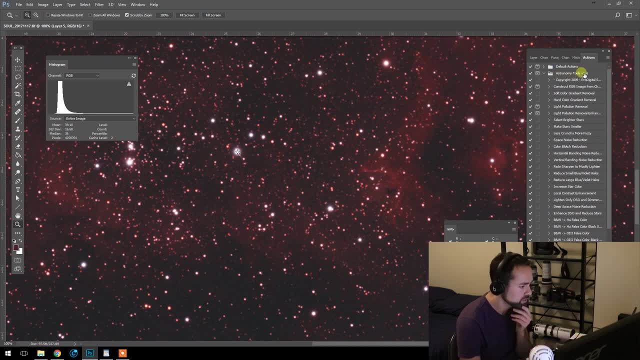 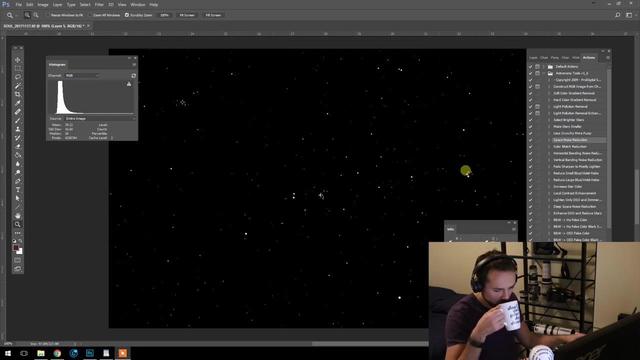 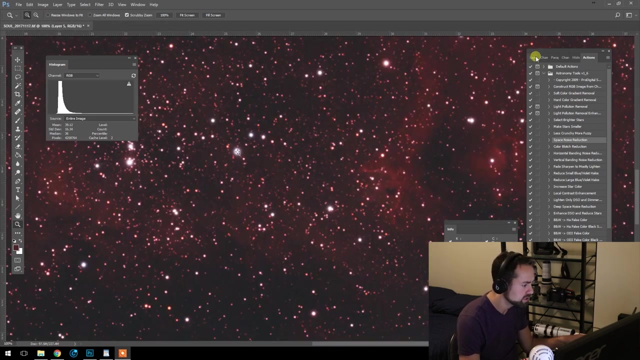 If you can see the folder here, Astronomy Tools, and the one we're going to use is Space Noise Reduction. Okay, So I'm going to run that Takes a few seconds And then, once that's done, we'll look at the before and after to see what that's in fact. 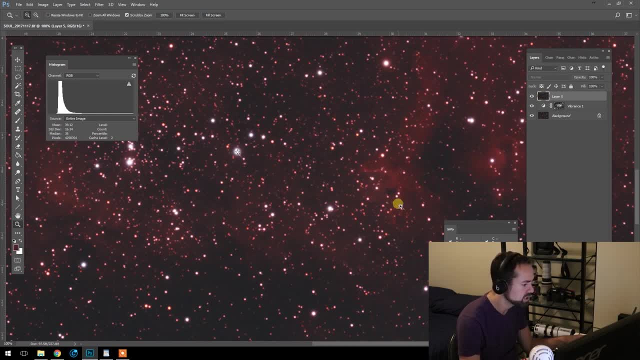 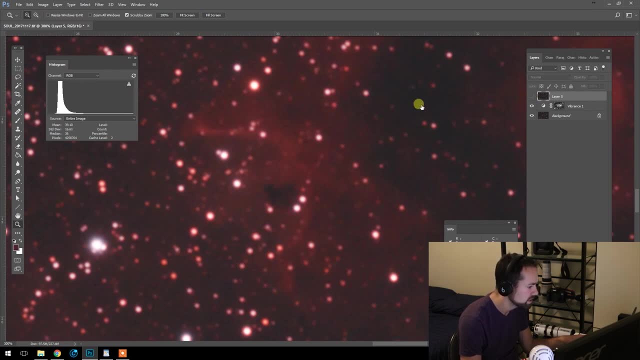 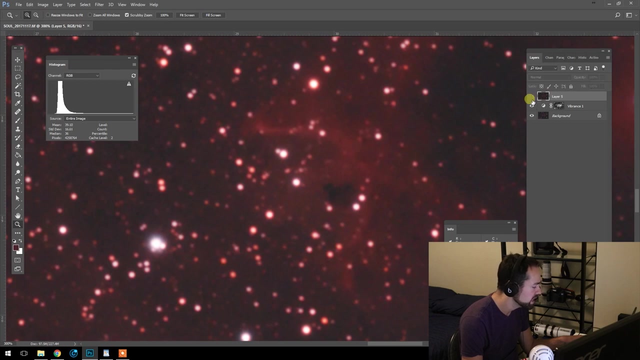 done And, as you can see, it does a great job. So let's look at this area here. zoomed in, That color noise that you can see has been fixed dramatically. You do lose a little bit of detail, though, but when that detail includes a lot of noise. 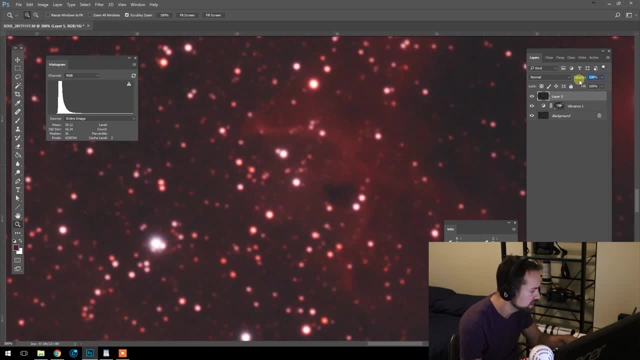 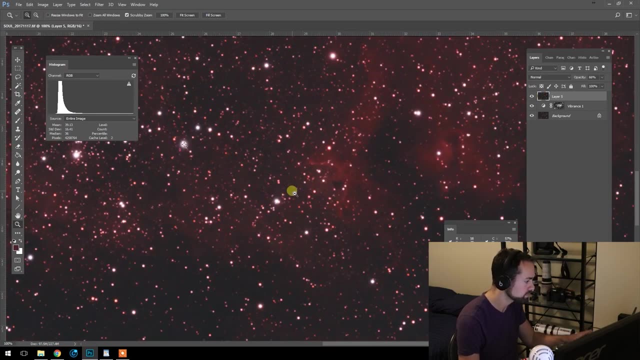 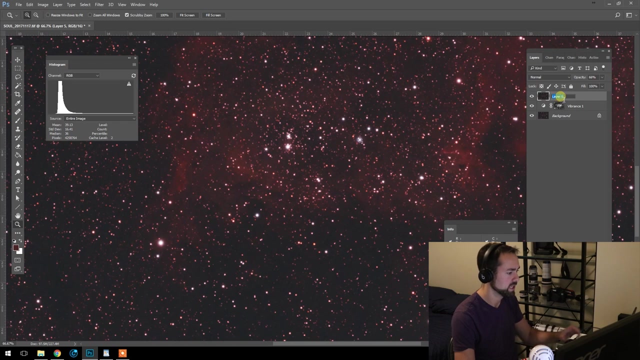 it's a fair trade. That being said, I think I'm going to use this, at about 66%, to try and get the best of both worlds here. Sorry about that noise, Okay. So now I'm going to do another level of another iteration of noise reduction. 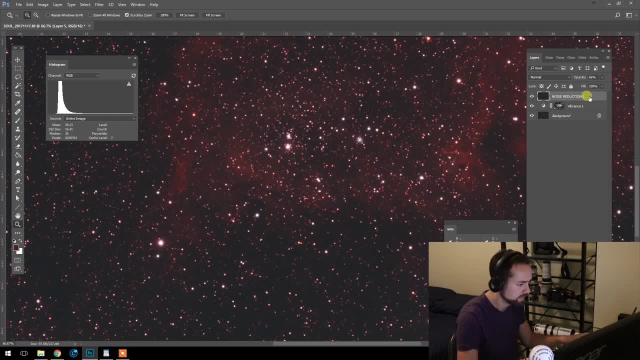 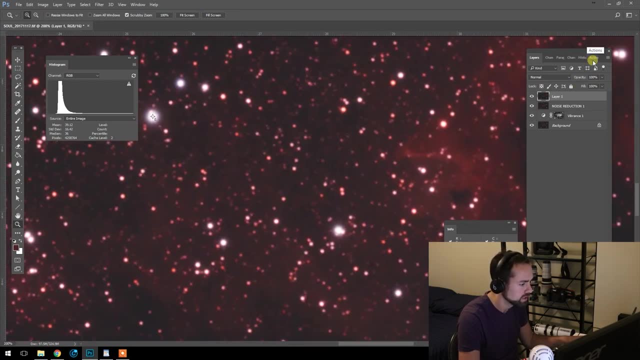 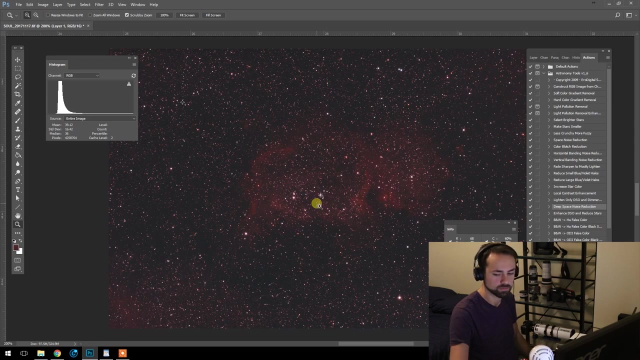 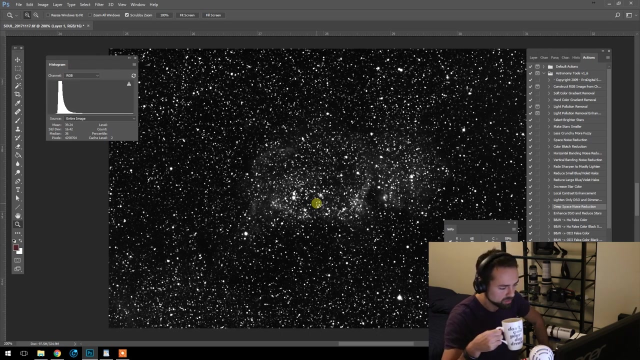 So we'll call this Noise Reduction 1.. And I'm going to create my new layer on top, And this time we're going to do Deep Space Noise Reduction. Now, the Deep Space Noise Reduction calms the darkest areas of the image, So it should make a difference to our background sky. 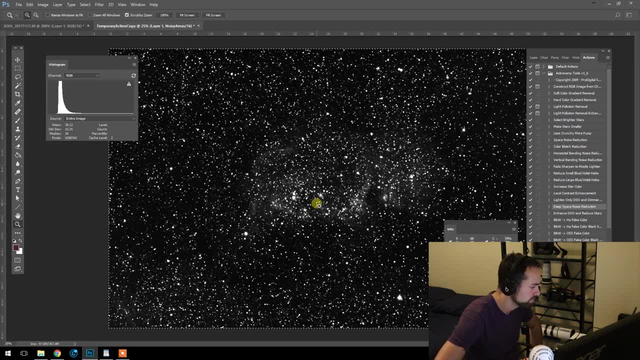 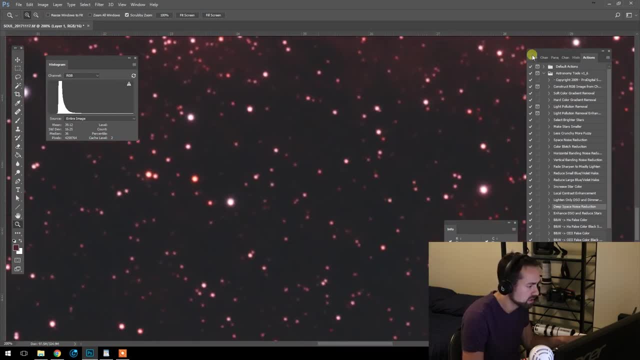 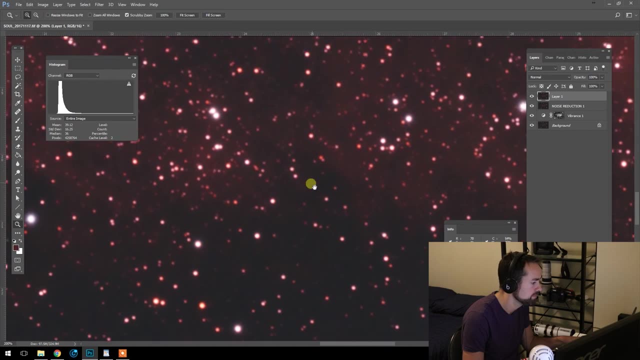 Another one you can use here is the Blotch Reduction action. That one does a great job as well if you happen to have some blotchy areas in your image. So let's take a look at what's been done here. So, as you can see, it kind of softens everything up but also gets rid of a lot of noise. 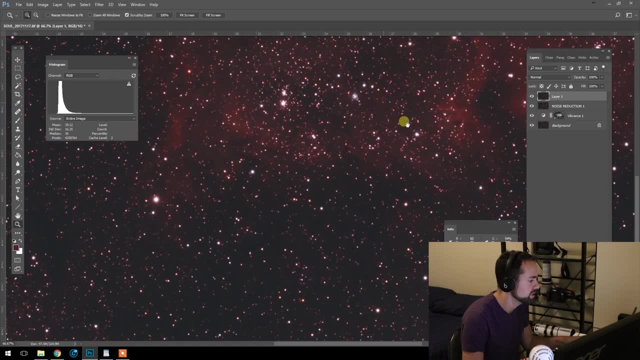 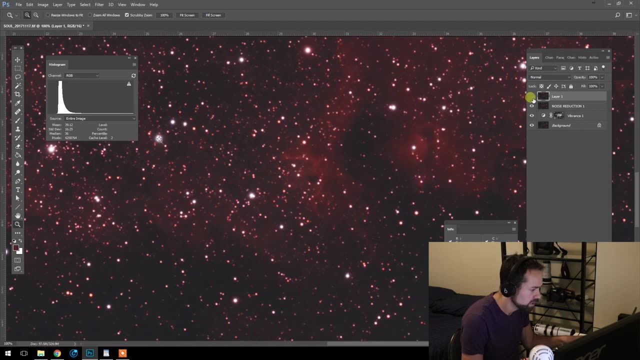 And that's a good trade off If you really just despise seeing noise And I feel like I have a higher tolerance than some. but for this one, why don't we just smooth everything right out? We lost a little bit of detail, but we can sharpen that up later. 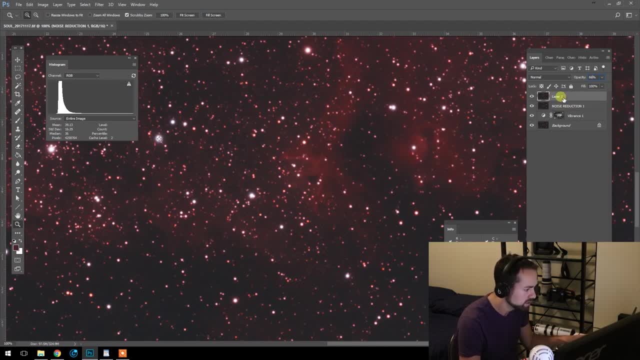 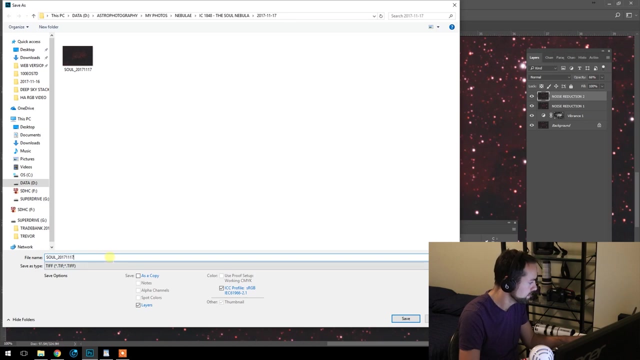 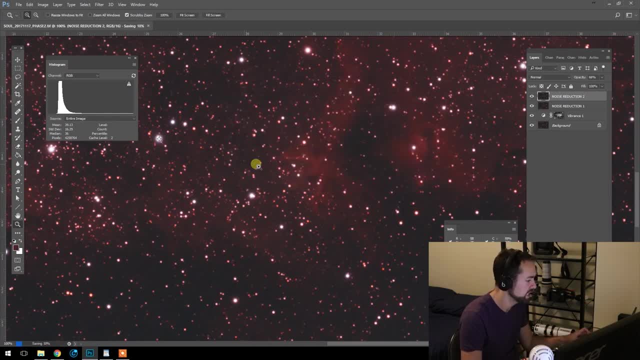 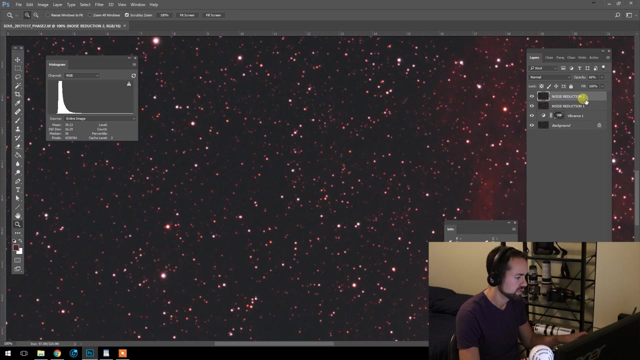 Whatever you want to call it, But it is nice to go back, and especially if you want to reprocess things. but you're happy with your first few steps. So that's Noise Reduction. At this stage I'm going to look at the color balance a little bit. 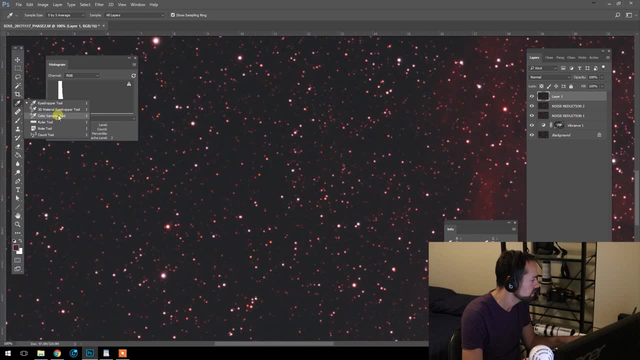 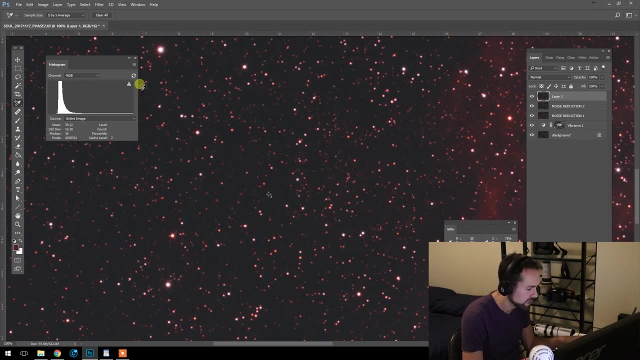 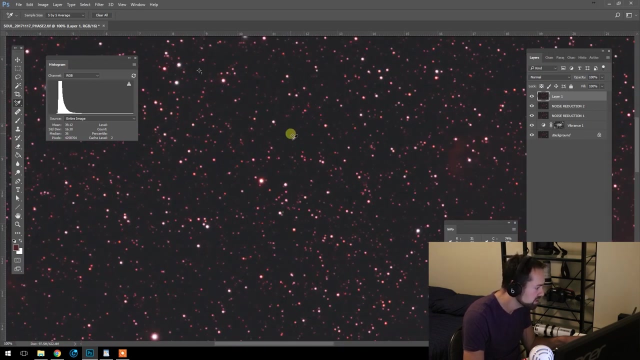 It's looking a little off in my eyes. Okay, So we'll set our color sampler in a smooth area of sky here, And yeah, it looks like the blue is a little high, which is surprising. Why don't we just use our tried and true? 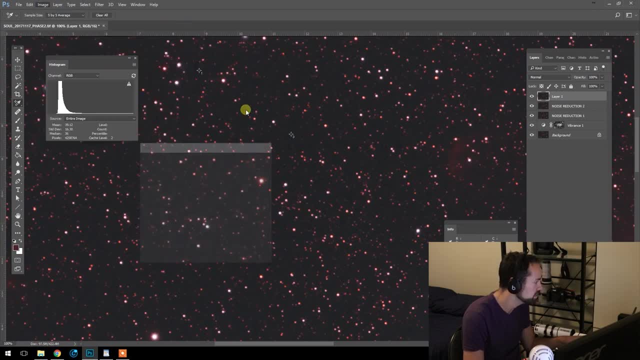 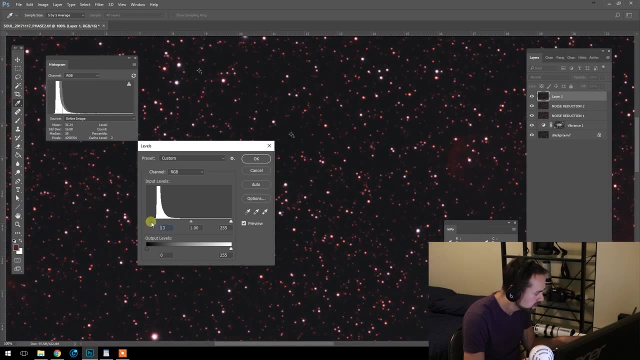 Actually this looks like a good spot. Yeah, again, the blue is a little high. Let's just pull everything in. So we're sitting at 26%, Okay, 24. 25. 28. Pull the green in. Like I said, a small change can make a big difference. 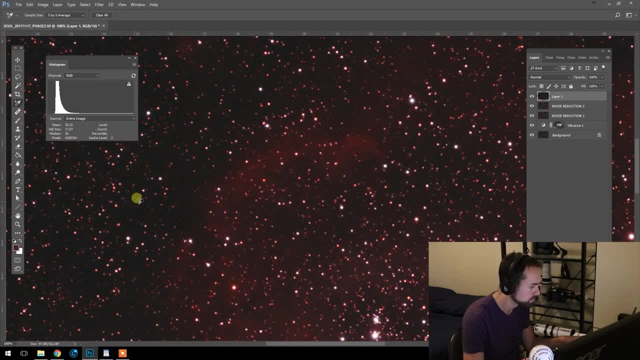 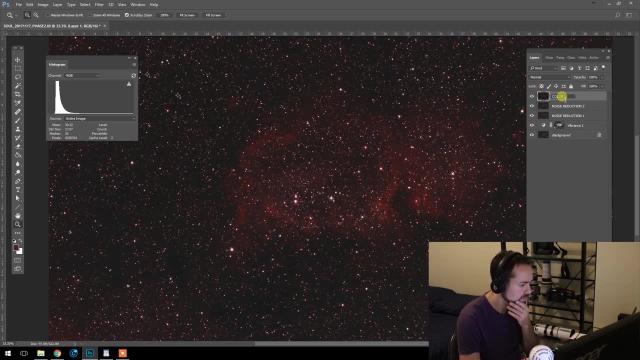 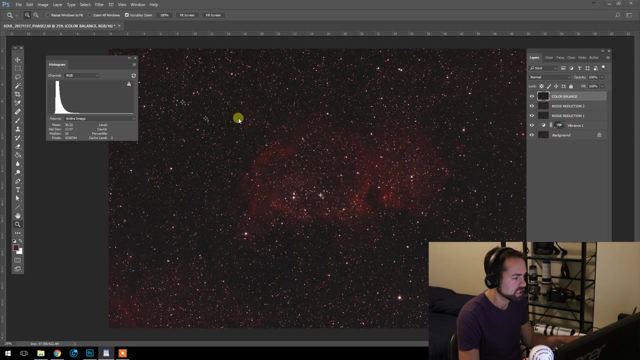 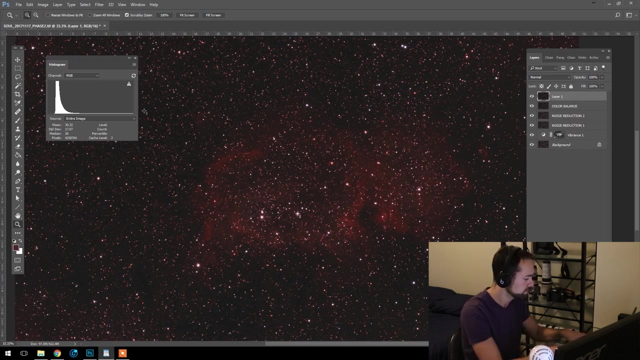 And the blue to 24.. Okay, Here we are. I'm quite happy with this. This is our color balance. Okay, And now we can work on sharpening One of my favorite steps. So we'll start a new layer. 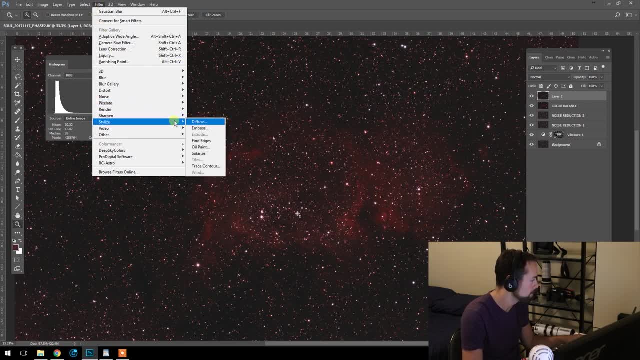 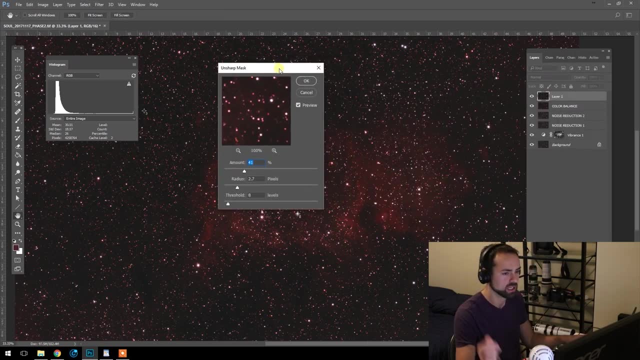 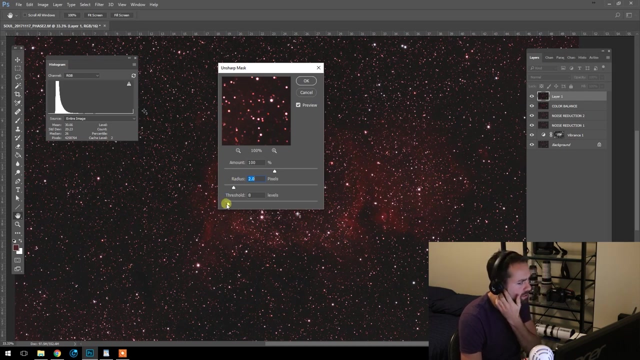 And we're going to use the unsharp mask. So under Filter Sharpen, Unsharp Mask. Now the settings I'm going to use here: The amount is going to be at 100%, The radius at two And the threshold at six. 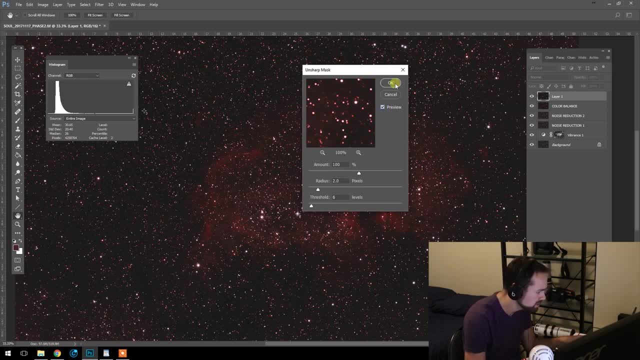 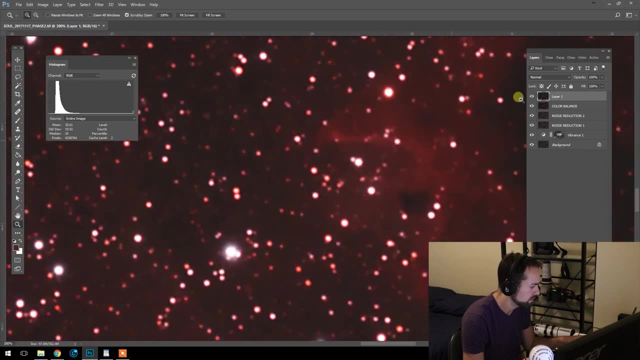 You can press this preview toggle here. Okay, And I've run that. So this is our sharpen layer. As you can see, it has sharpened the details slightly, But it's also created the halos around the stars. So there is an action that helps with that in the Astronomy Tools action set. 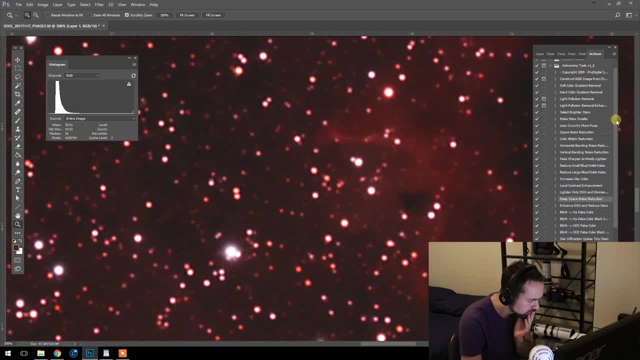 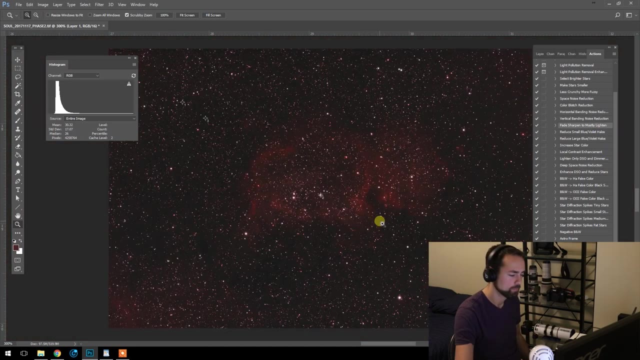 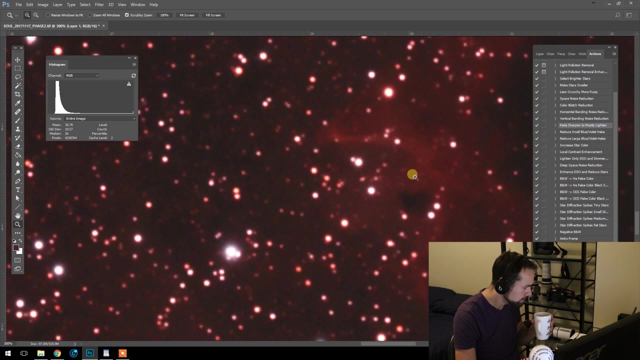 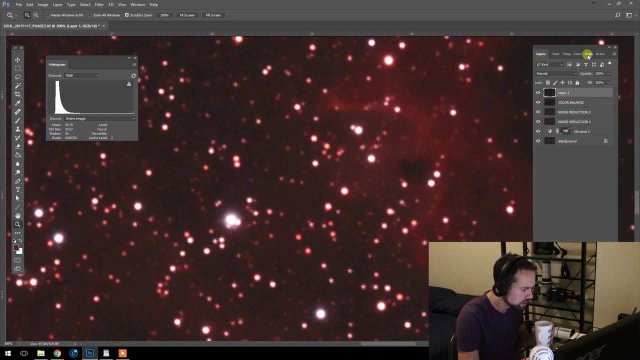 And it's called Fade Sharpen to Mostly Lighten. Let's have a go at that. If I could find it. There she is. I believe it did help. I believe it did help. So we'll have to go back to our history here. 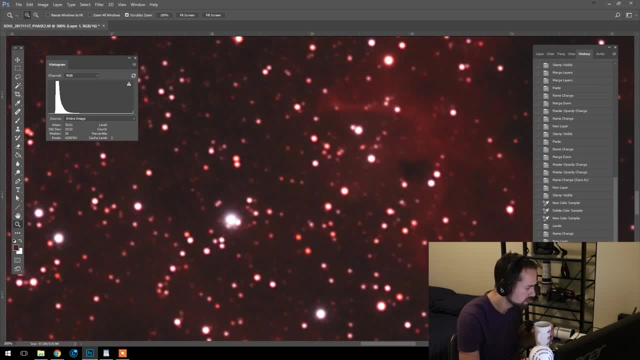 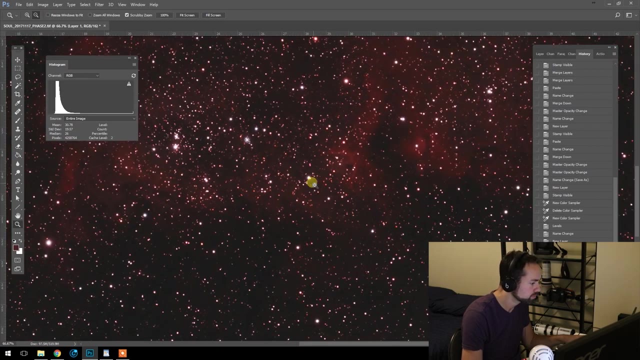 Because I didn't make a new layer. So Unsharp Mask, Fade to Wow, It really helps. Fade Sharpen to Mostly Lighten Holy smokes. That helped really well. So let's look at our sharpen layer here. 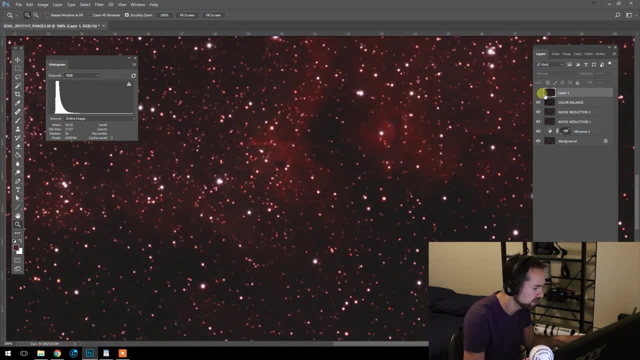 Before and after. So this is kind of a good area to look at. Okay, So It sharpens the details, but it sharpens the stars as well, And that's not necessarily a good thing. I like the stars to have kind of a soft edge. 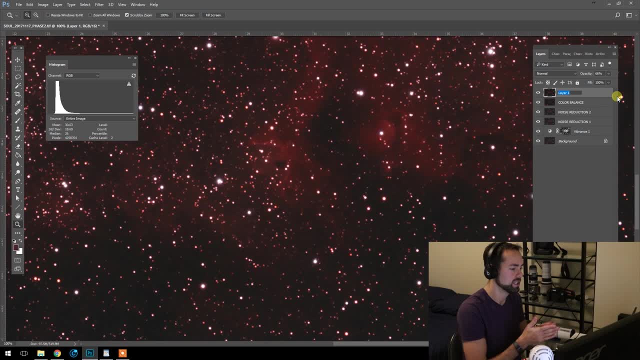 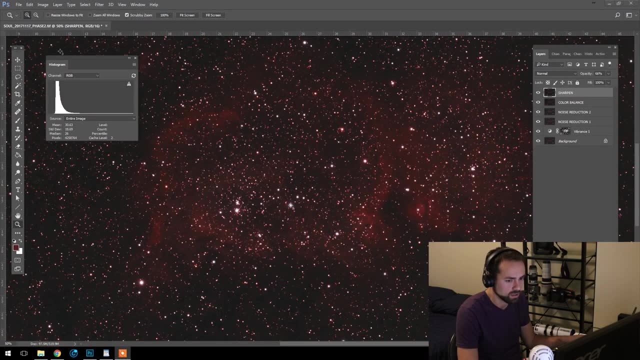 So again, When in doubt, Do it in thirds. So I've got 66% sharpen, Alright. Now we are getting closer to finalizing our image here And we are going to minimize the stars. This makes a big difference in the image. 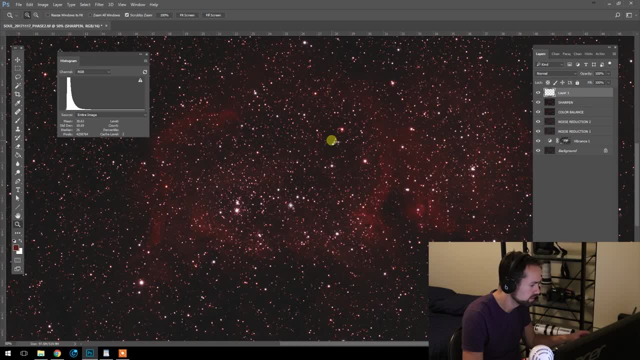 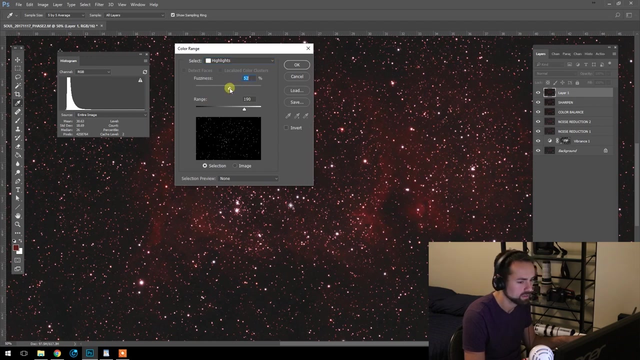 So let's create our new layer here. Again, that's Shift Control, Alt N plus E, Select color range, And this time I'm going to do highlights So you can adjust this fuzziness slider. I've got the range here at 190.. 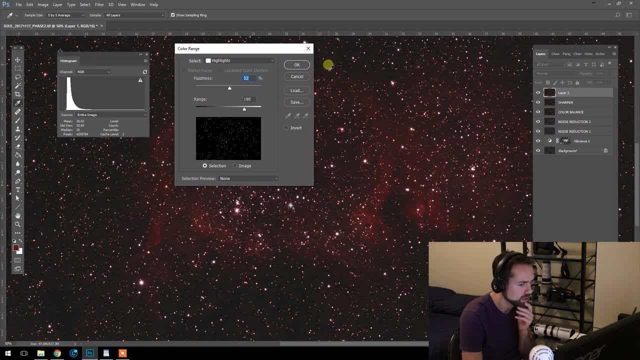 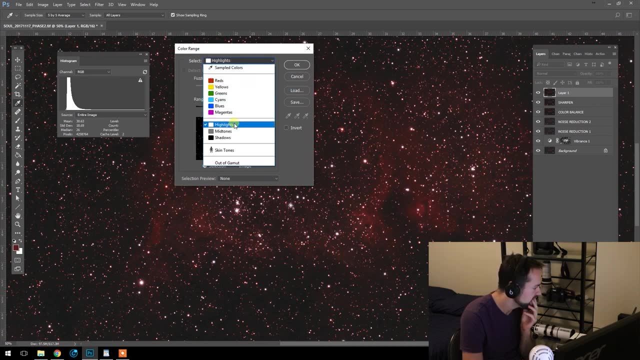 Um, The other way you can do it Is to use sampled colors On the eyedropper- on a star, of course, Rather than highlights. Um, Let's see if that's any more accurate. So I've got the biggest and brightest stars here selected. 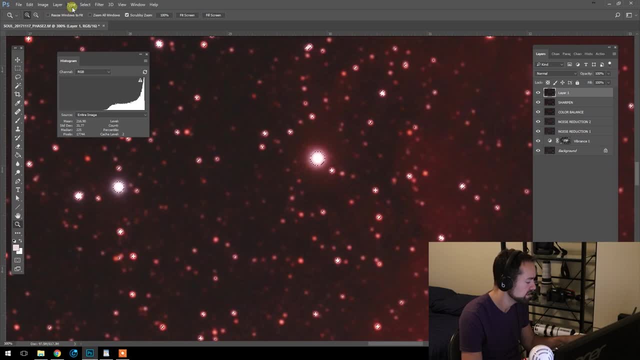 And, As you can see, It's only got kind of the inside of the star without the outer halo. So we are going to go to select, Modify, Expand, Let's see about 3 pixels. You just want to get the entire halo of the star as well. 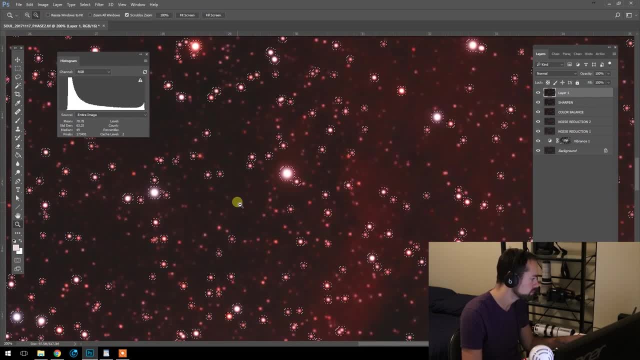 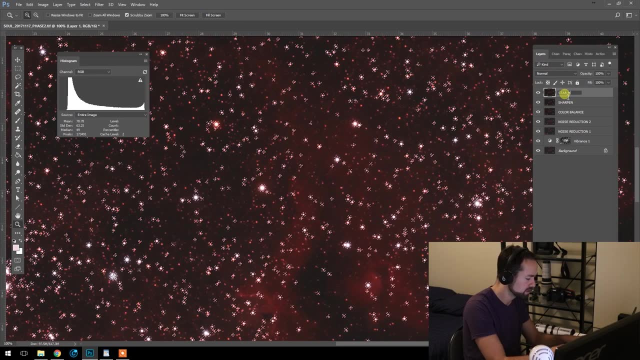 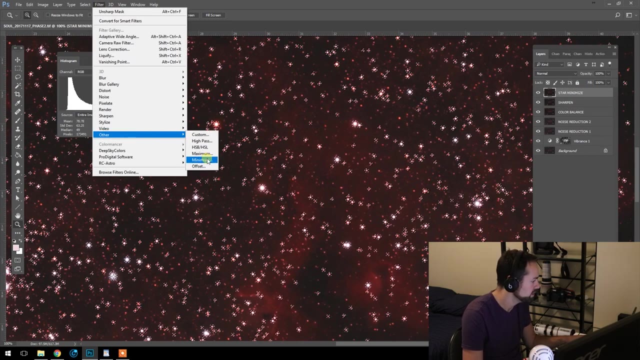 Expand by 1.. Here we go, Uh, This layer We are going to, Before we forget, We are going to name it Star Minimize And we are going to use filter Other Minimum, And we've got a radius of 1.. 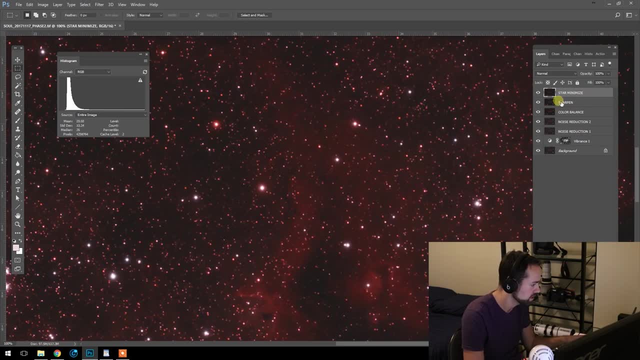 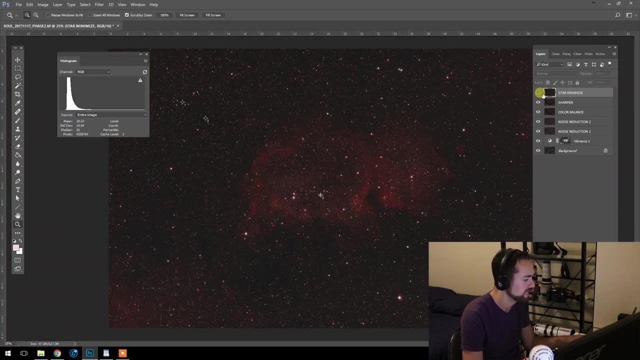 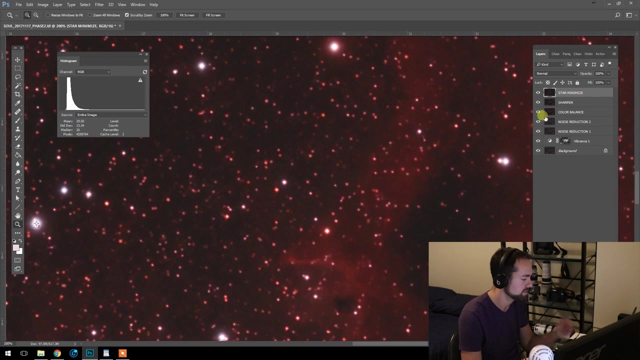 It's giving us a little preview of what it does to the stars there. Very powerful technique. What a difference, Right? And when you reduce the stars like that, The object shows up that much more. It kind of pops from. It's not hidden behind all those bright stars. 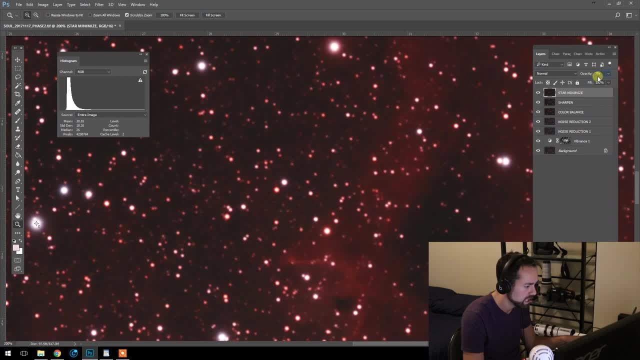 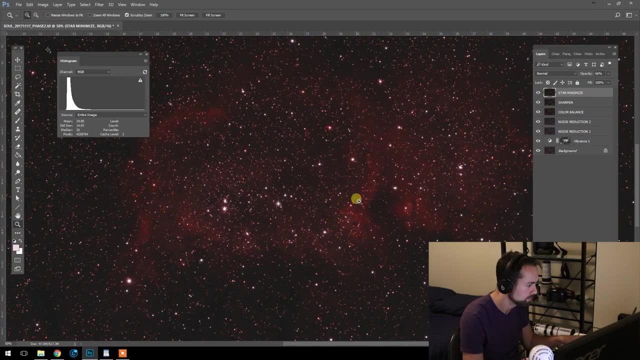 And of course That's a little drastic for me, I'm going to set the opacity to 66 percent. It's done a great job at making those stars smaller, But it's left it still a little bit more natural than if we left it at a full 100 percent. 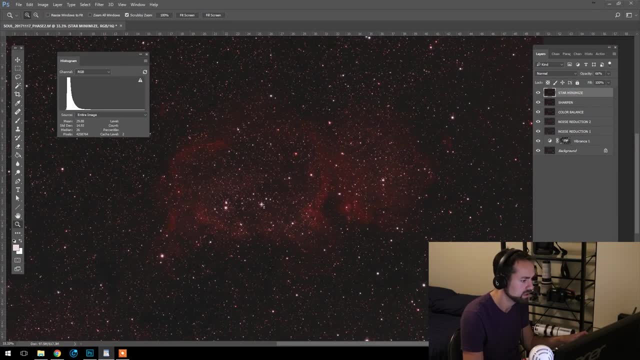 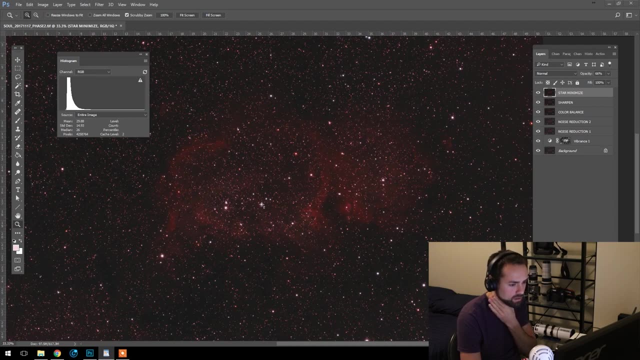 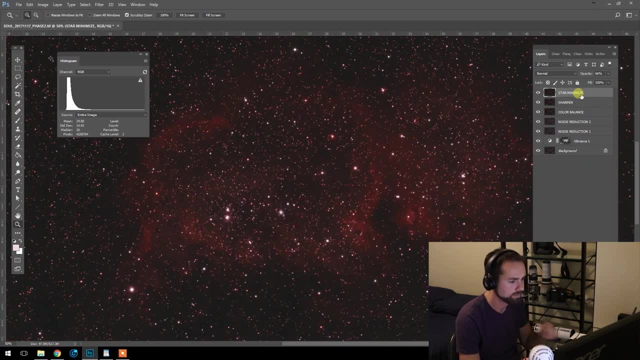 Let's see, Let's see, Let's see. Okay, Okay. Another way I like to do it is using the astronomy tools action set. It's one of the actions I use in every single one of my photos. Very powerful, I'm going to create a new layer on top. 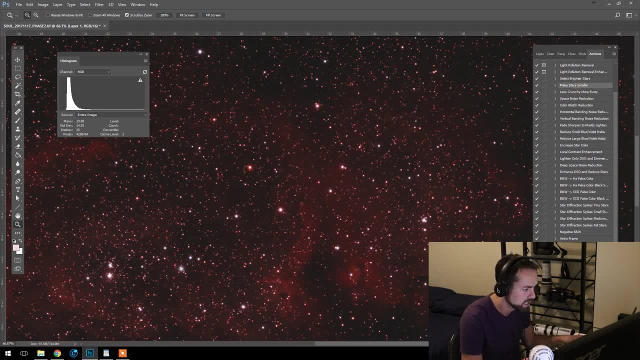 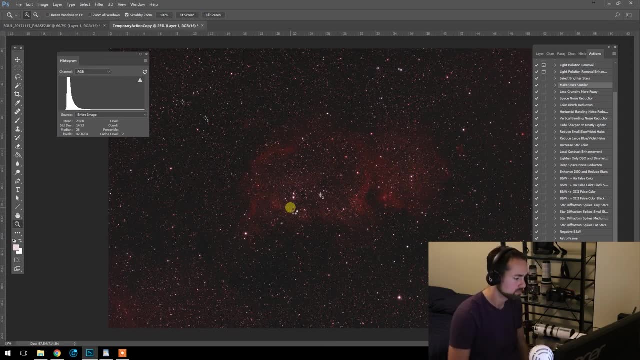 This time we're going to go into the actions And go to use the make stars smaller action. This can be run several ways. This can be run several times, but it's easy to get carried away and not realize what it's actually doing to your stars. 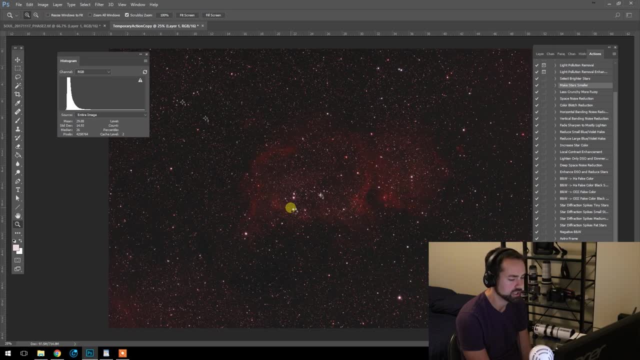 They can start to kind of morph into each other and kind of show up as diamond shapes. You don't want that. So pay attention to the quality of your stars while you're. don't get too carried away with just the contrast of your nebula. 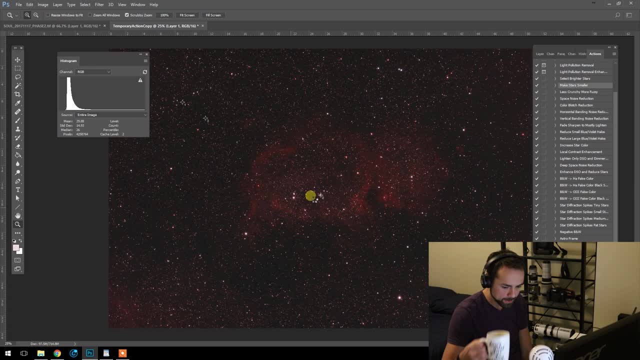 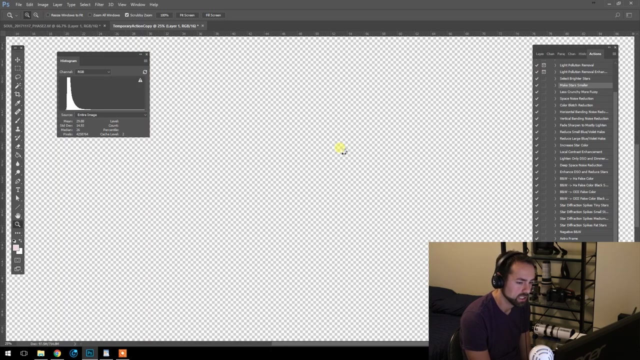 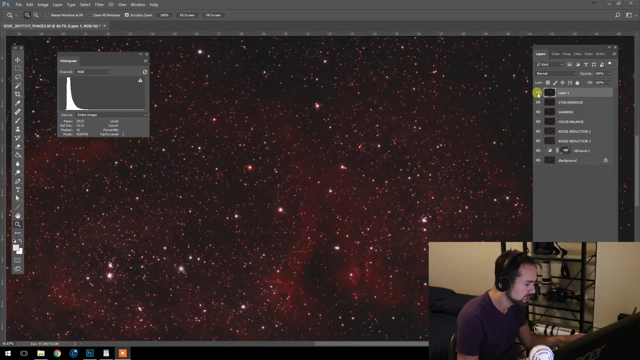 Pay attention to those stars. That's the progress bars on my other monitor here running Still going. You think this is long wait till you see how long it takes for the next action. The make stars smaller action has finished. That took a while. 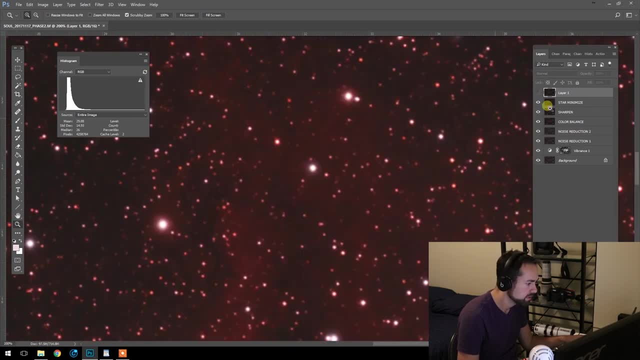 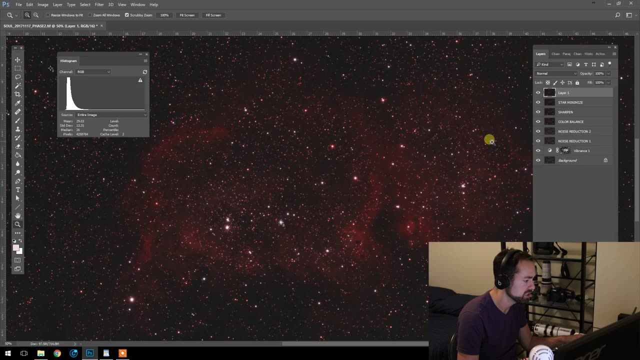 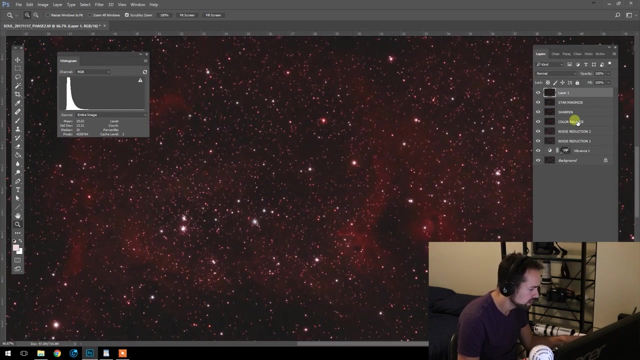 So let's turn it off and on, as always, to see the difference. So that's without it and that's with it. Subtle, but just does a beautiful job. If you can see, this is starting to look very nice. Just to save my computer. 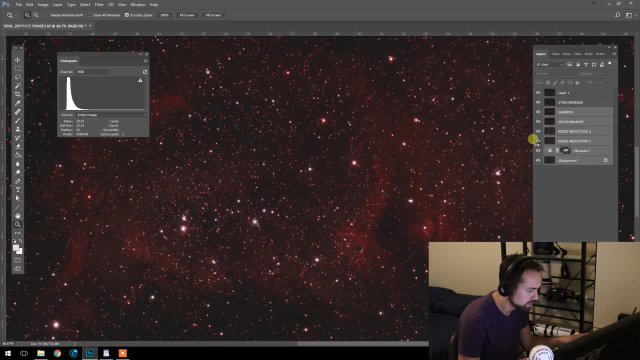 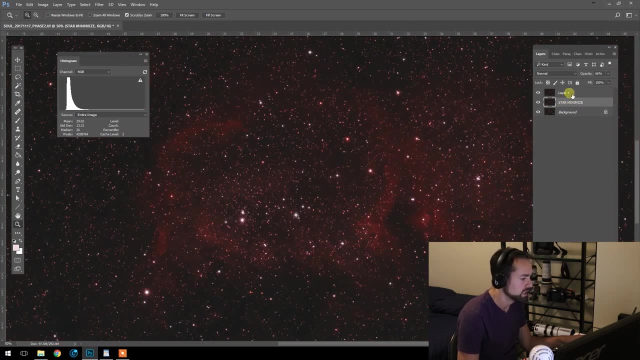 I'm going to merge these layers all together. If you don't mind a huge file size and you want to go back and make changes, you'll want to keep those layers in there. So we'll call this layer star minimize two, And I'm really loving the way this is looking right now. 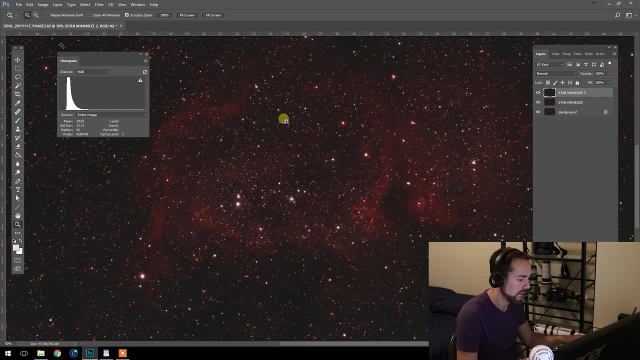 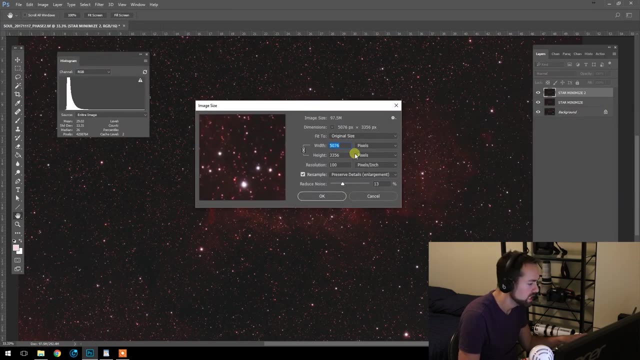 So the next action? I'm almost scared to run it. It's going to take a long time. This image is- we haven't scaled it down at all, So I mean it's 5,076 pixels wide. It's a nice large image. 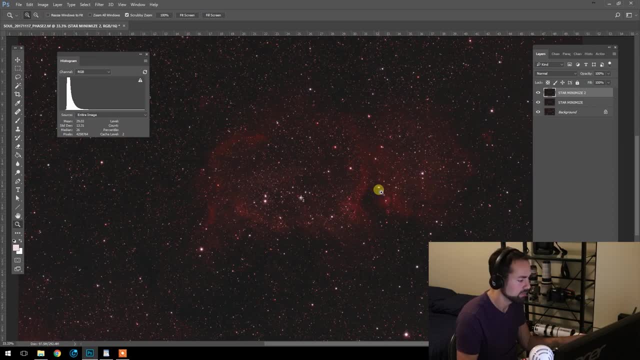 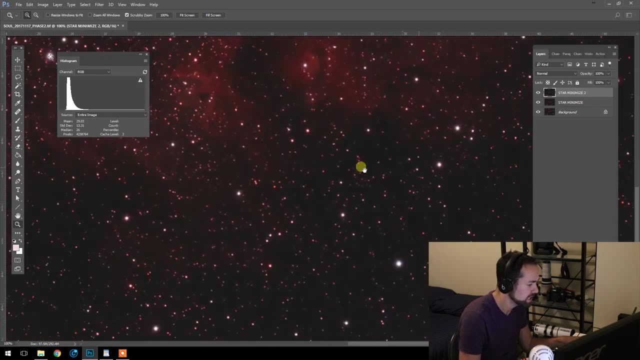 which is great that it's looking this good at this size. We could print it out poster size, It would look great, Or just a high resolution photo online. I mean at a hundred percent it's you can, you know. 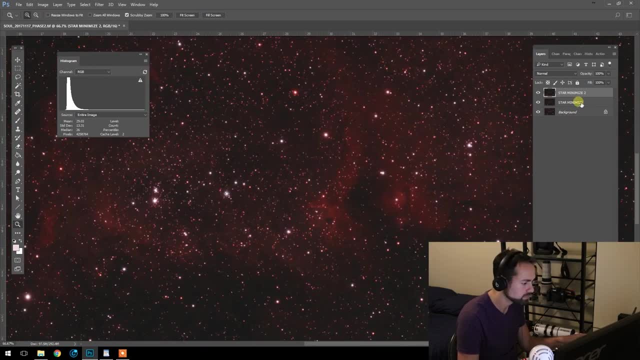 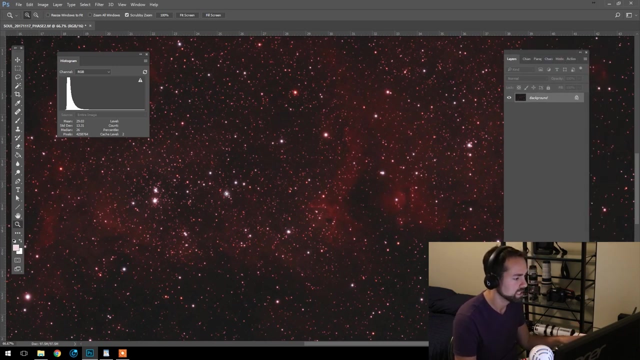 kind of look around and enjoy it, Enjoy the scenery. I love it. So the next action- and I'm literally going to merge everything together for the purposes of this tutorial- This is: this is throwing my non-destructive workflow out the window. 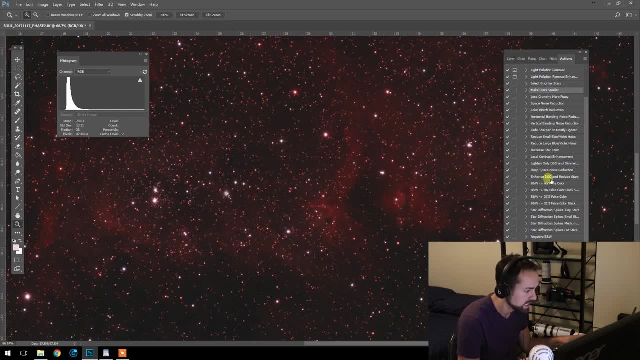 So the action I want to run here is called enhance DSO and reduce stars. Again, this is one that I use in every single astrophoto and it's basically it really works like magic, So it's going to pull forward some of the dim details. 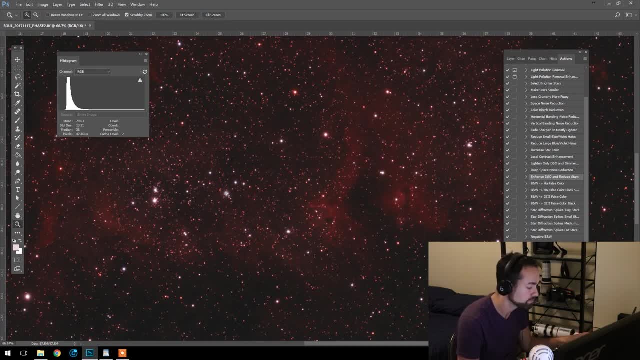 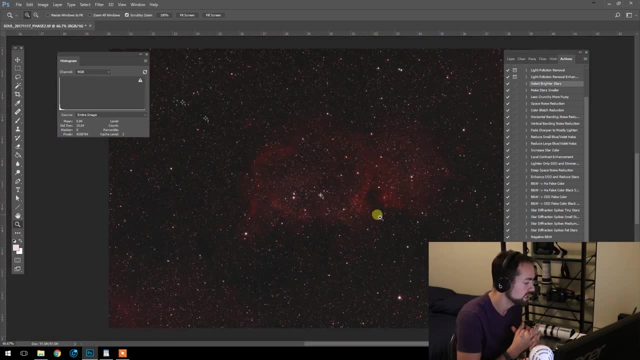 of the nebula and reduce that star size even further. So I'm going to run this now and then I'm going to go refill my coffee And this might take up to five minutes on this image. See you in a minute or two. 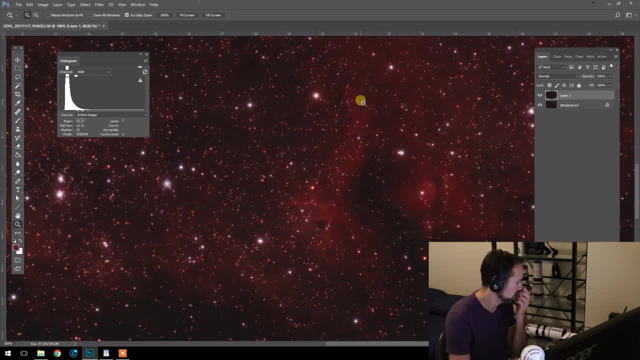 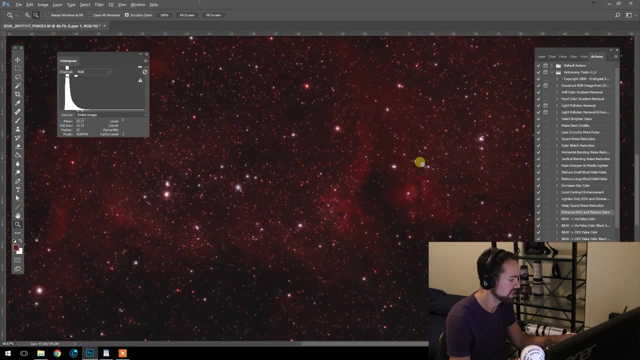 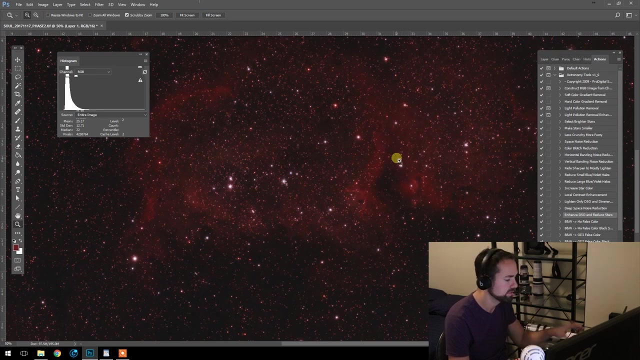 So the action has completed the enhanced DSO and reduce stars in the astronomy tools action set. It's an extremely powerful action. I love what it does to my astrophotography images. It's one of the reasons I love this action set so much. 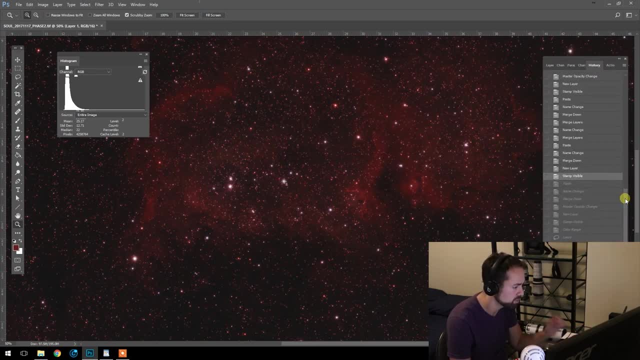 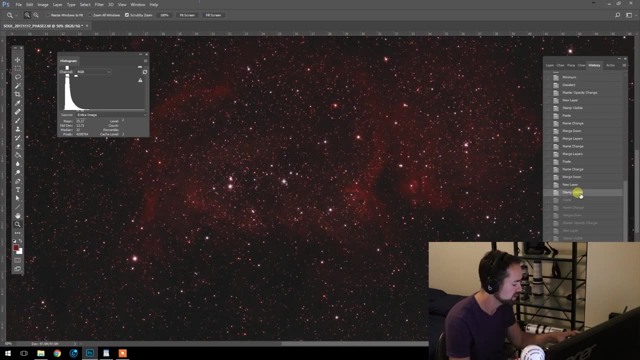 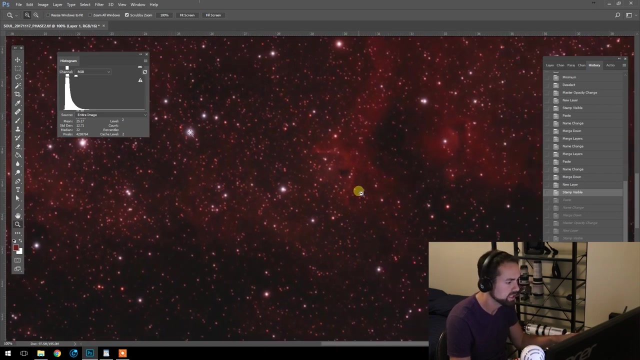 because I flattened everything to speed things up. We have to go back in the history to see it before and after. So this is this is before the action was run and this is after. So very powerful. I just love what. I love what it does to the image. 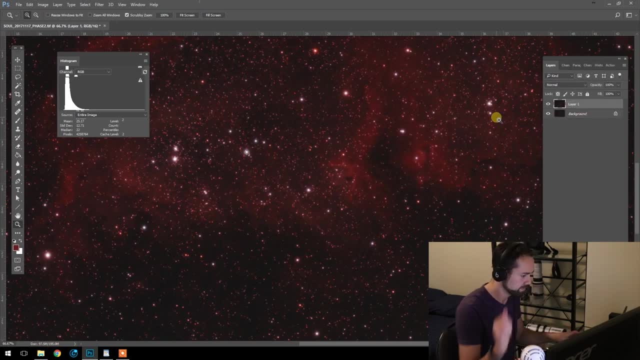 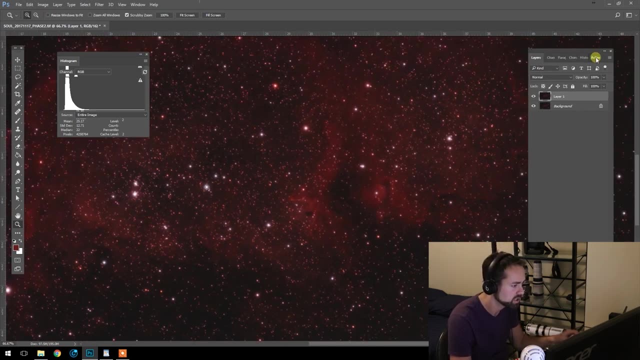 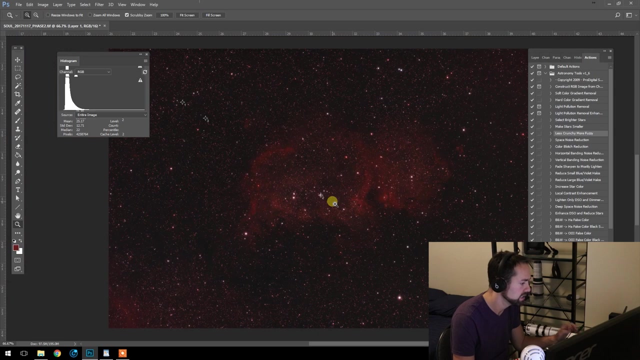 So we're going to move on from here. I've created a new layer on top, I've stamped visible and now we're just going to run a quick action called less crunchy, more fuzzy. Now that's going to soften up the stars a little bit further. 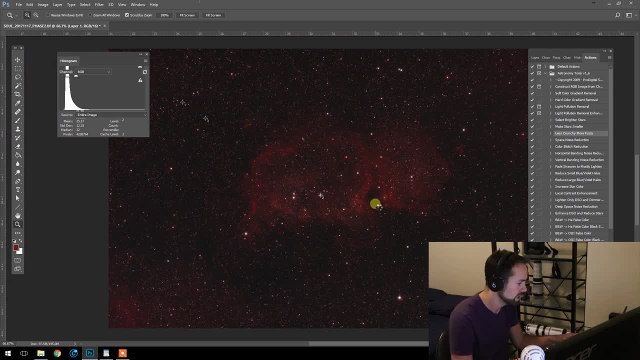 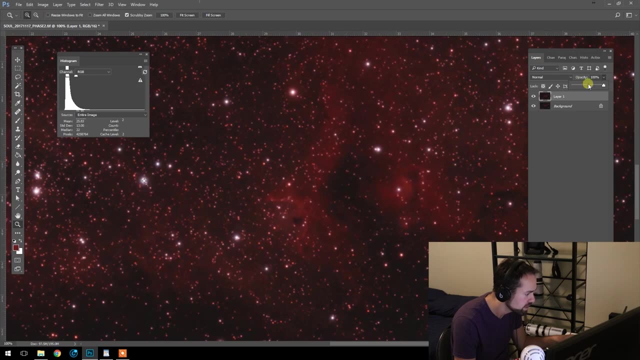 It's going to sharpen our details as well, but there's some things we can do about that afterwards And, of course, we can adjust the opacity of this, this layer. So the before and after. look at some of these smaller stars here. 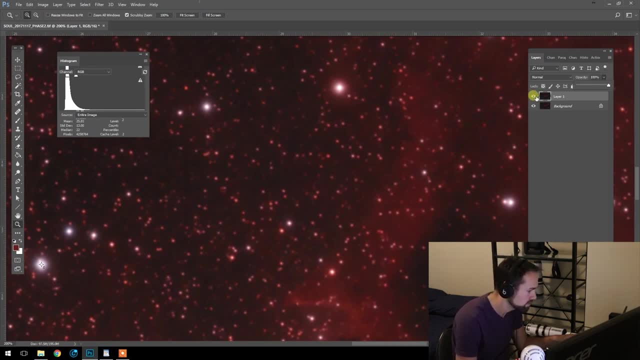 Let's turn this up to a hundred percent. So that's, this is before: the less crunchy, more fuzzy, and this is after. So you know it makes them look like glowing orbs, as they are as opposed to, you know, crunchy, crunchy dots. 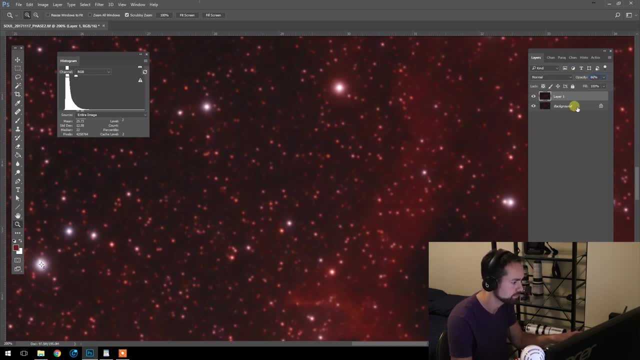 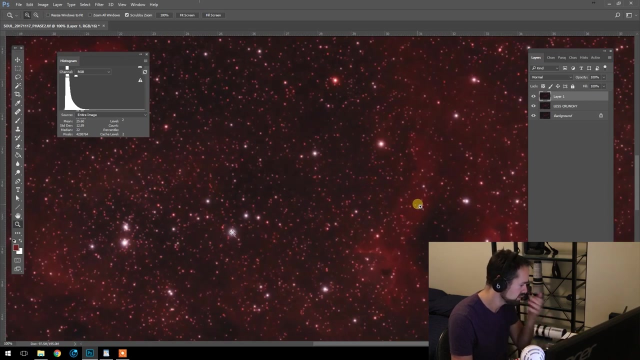 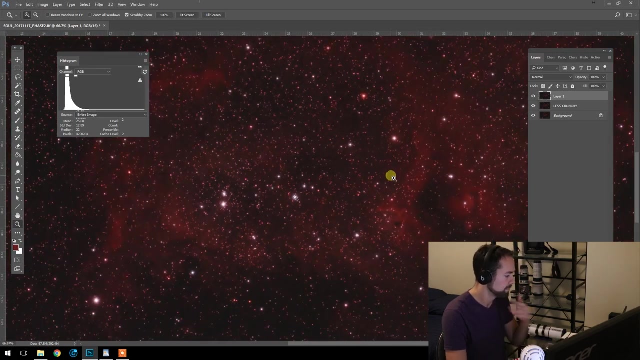 So I like that one. I'm going to leave it at 66%, Less crunchy. And again, you would have all your original layers in the layers pallet here. Your file size would be huge, but at least you could go back. All right, sir. 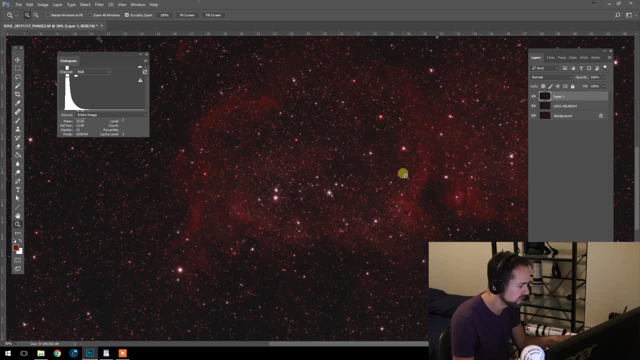 So the next step would be would be to do some selective sharpening, And I'm going to be doing that kind of i like to do it, but, who knows, maybe you'll like doing it this way too. so, with our layer on top here, 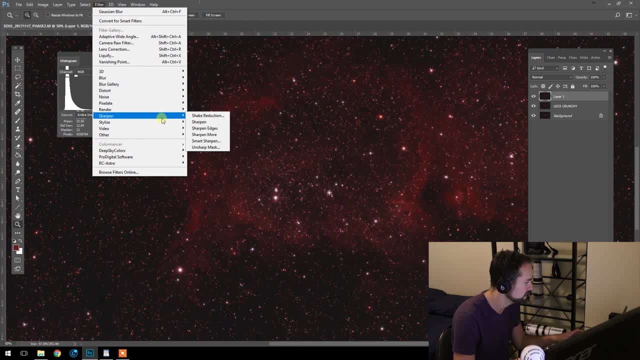 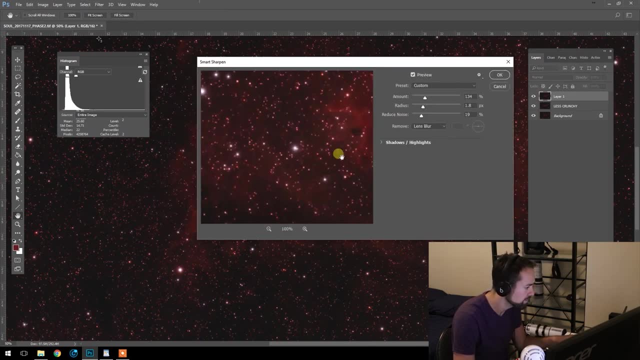 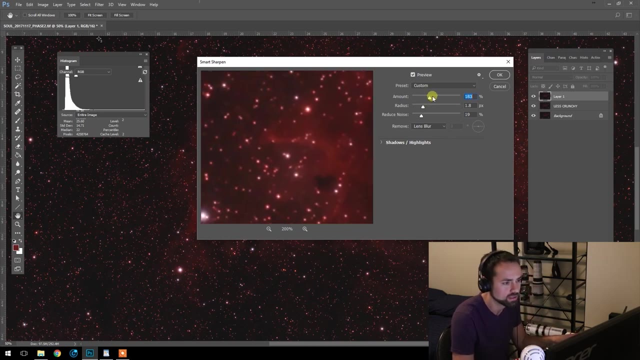 i am going to go into the filter sharpen, smart sharpen, and in the preview window i'm going to go into some of the details of the nebula here and let's just see what we're going to do here. so you can, of course, play with these. i'm going to keep the noise reduction. 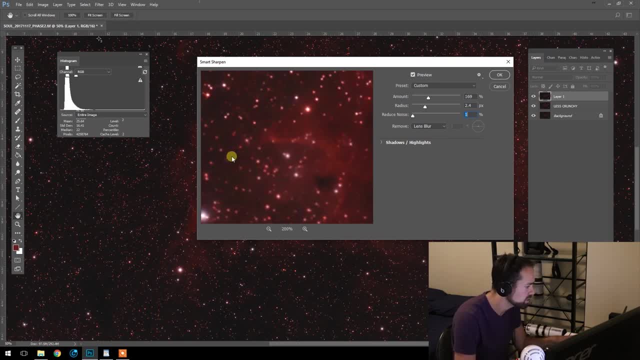 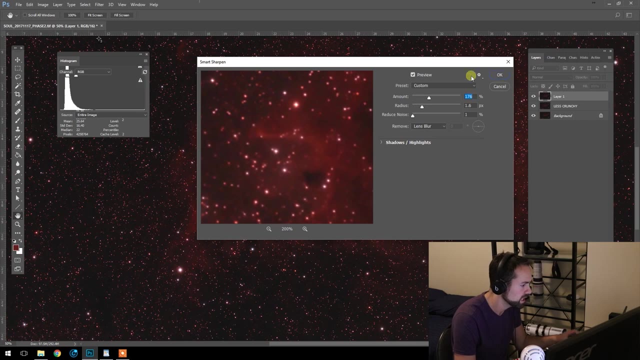 rather low and we're. the thing we're looking out for here is not to create too many of these. um, you can see these bright, red, hot pixels and we're actually just sharpening small stars and actually some noise in there, so you want to be careful with this. 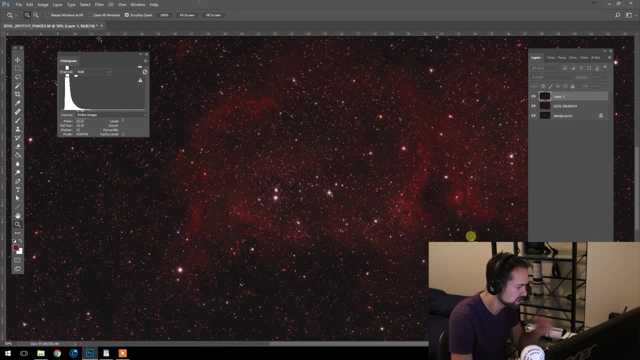 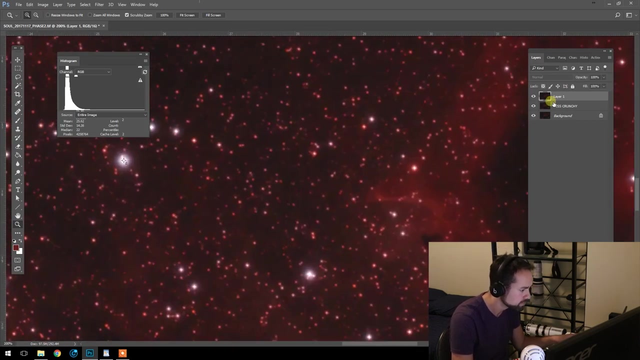 but bear with me here. so we'll run this sharpen on this entire layer here and it's going to crunch up all our stars and everything we've worked so hard to get to. but the key is so i'm creating this layer of before we did that and i'm going to put it on top of the sharpen layer. 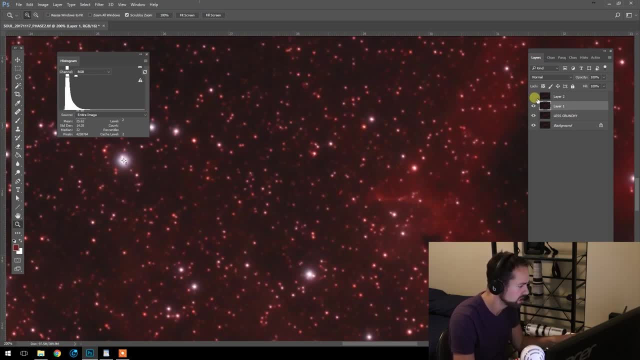 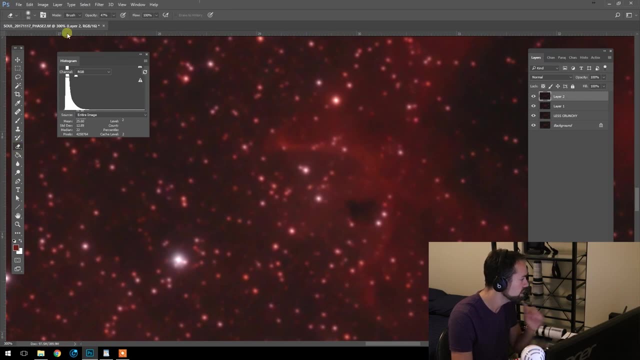 so when we, when we turn these the regular soft layer off, underneath it is the sharp layer. so with the soft layer selected we can go in with the eraser brush on, pick a good size hardness all the way down so it's nice and soft and then selectively we've got the opacity here. 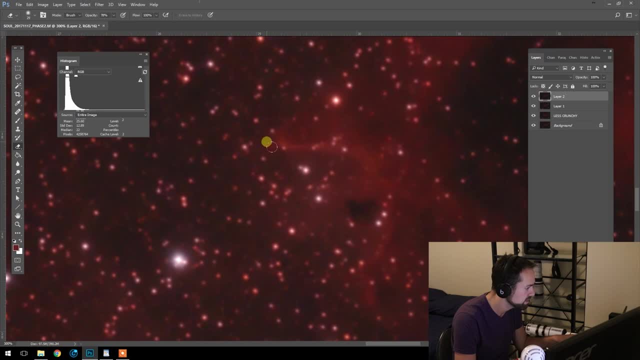 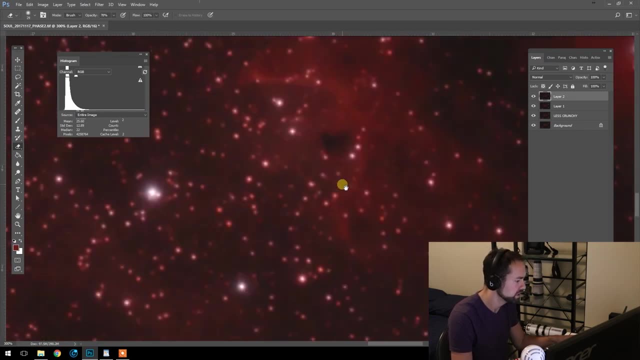 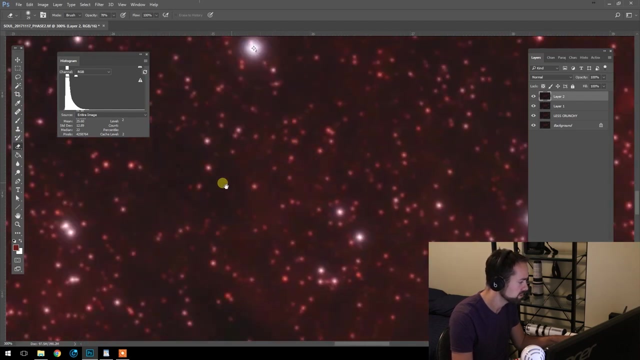 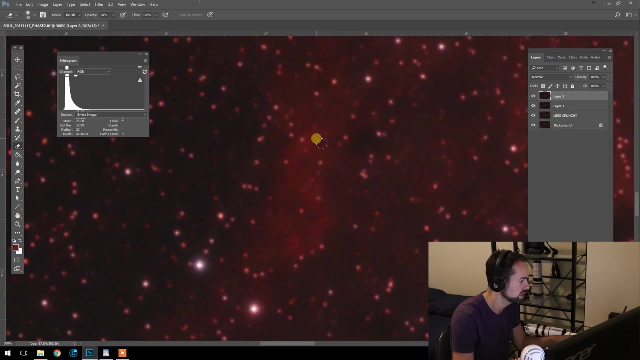 we'll turn that right up to about 80%, selectively erase this top soft layer and reveal the sharpness underneath. it's basically a mask. i prefer to do it this way with the layers in actual not using working from that mask layer, but actually just revealing the the image underneath. 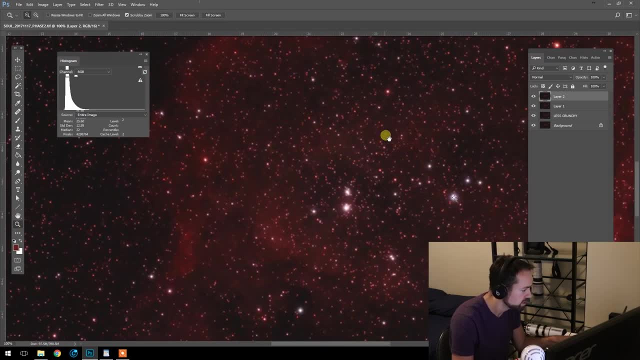 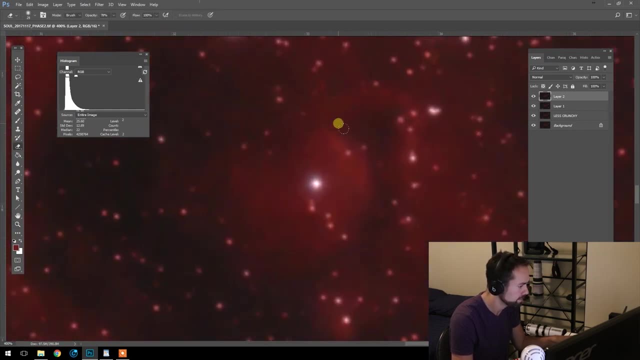 so let's kind of get a bird's eye view here. there aren't too many areas that i want to selectively sharpen like that. this would be one. so we get those, those hard edges of the dark dust there. subtle difference, but um, in the end it will make it'll be a noticeable difference. 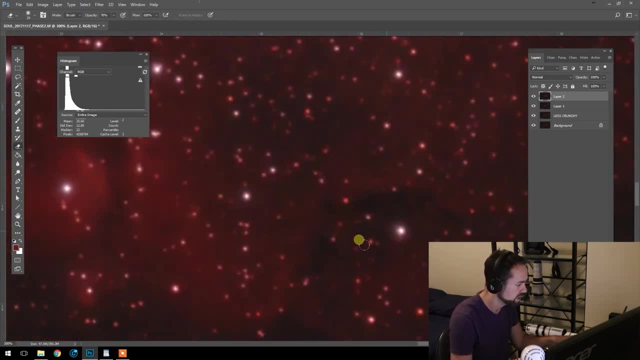 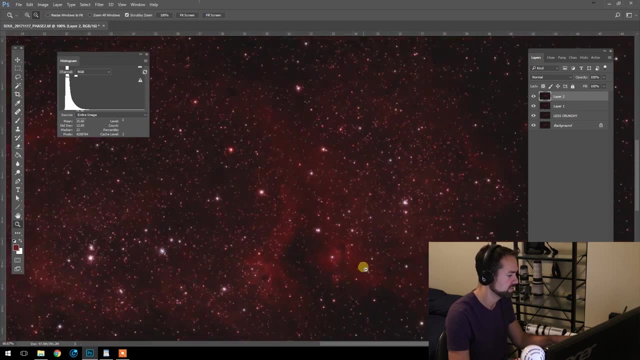 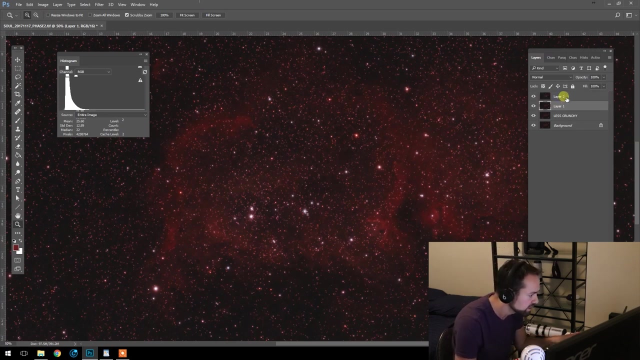 again here, being careful not to, you know, crunch up any of the stars, but this is something i do in a lot of my images and it really makes them pop. so if you see those sharp areas, chances are i've done some selective sharpening like this, very subtle in this one. um, i just thought i would show you that. 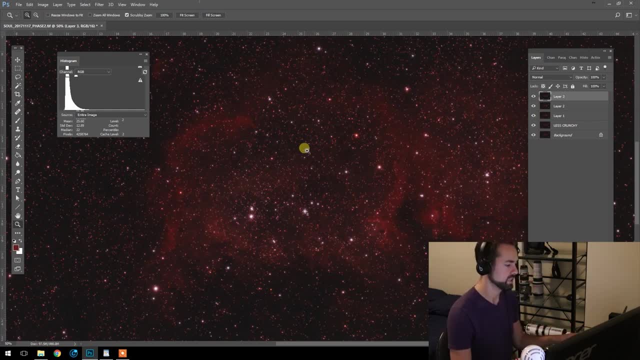 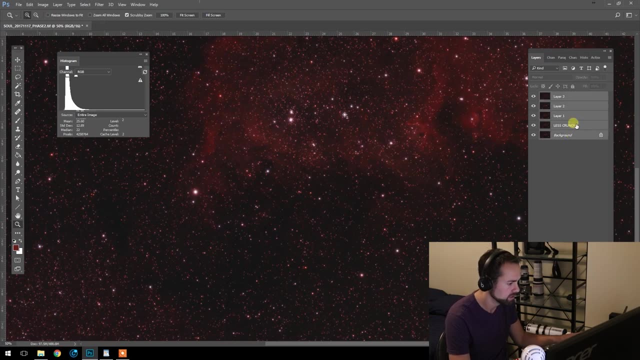 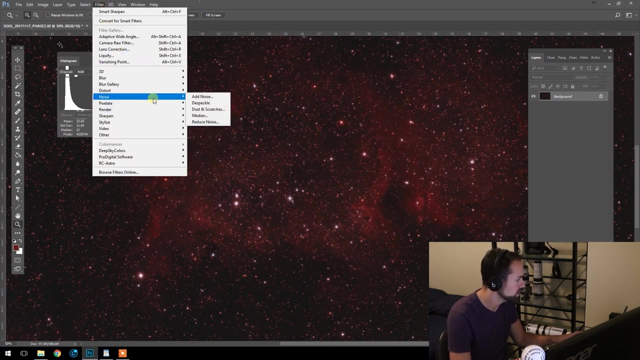 so that's just some additional selective sharpening. we've done so. the same way we've done that selective sharpening, we can do selective smoothing. i'm going to merge everything for the purposes of the video, this tutorial. so we're gonna go into, at least create one new layer. I'm gonna go. 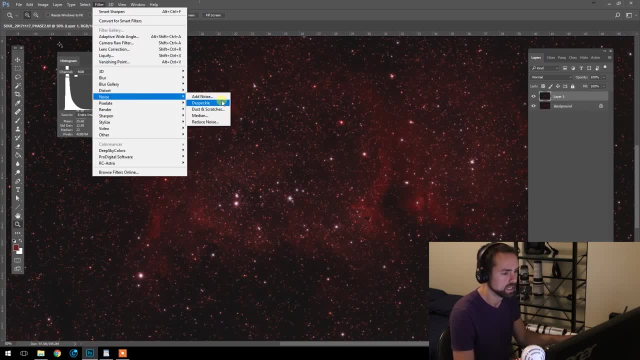 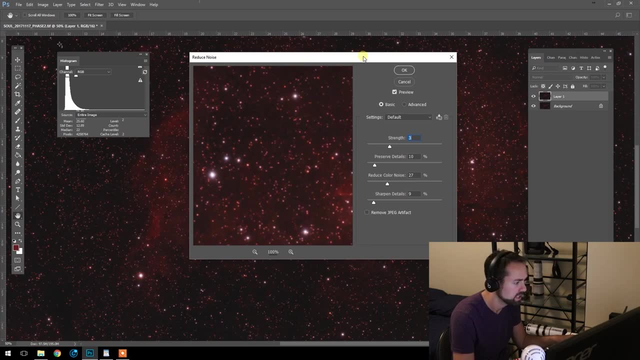 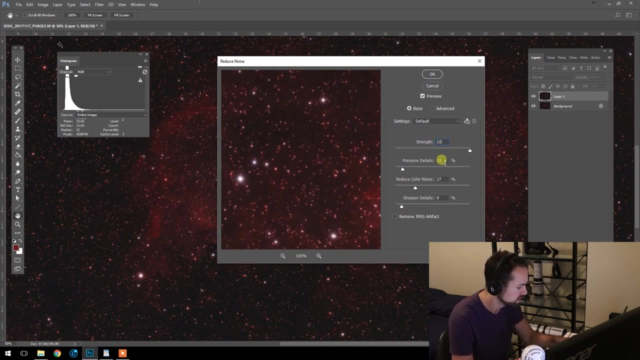 into noise reduction. reduce noise. this is just a standard filter from Photoshop and the settings I've got here. strength of 10. this is going to be pretty aggressive. preserve details of 90. reduce color noise. I'm gonna leave that 25 and sharpen none. so this is going to soften everything up. of course we don't want to. 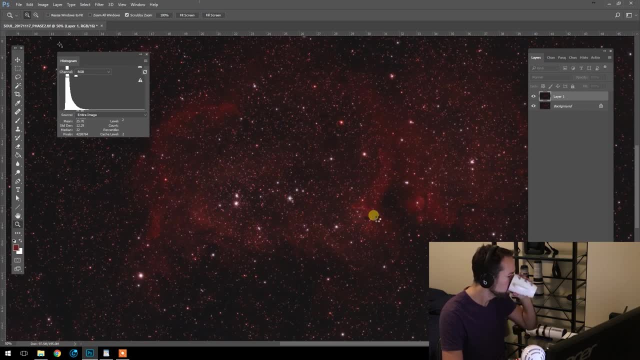 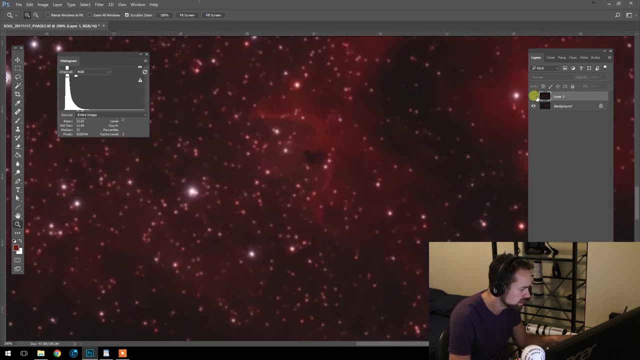 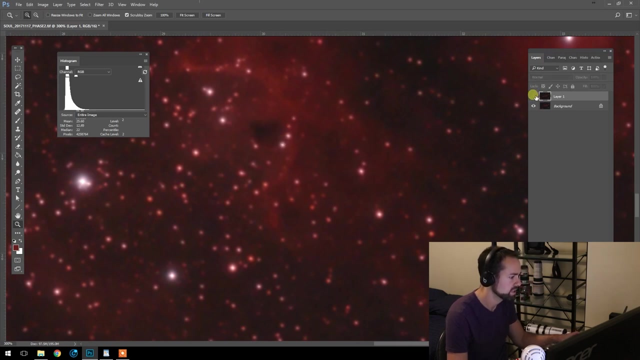 we're gonna have to remove the areas that we want to keep sharp. so if you can see the before and after, it cleans up a lot of the marry pad呗. this color noise here, but then it softens all our details there. so, the same thing, like before, I'm copying my, my background layer, I can put it on top of 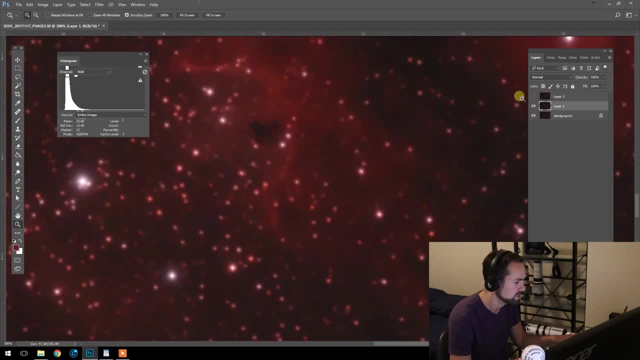 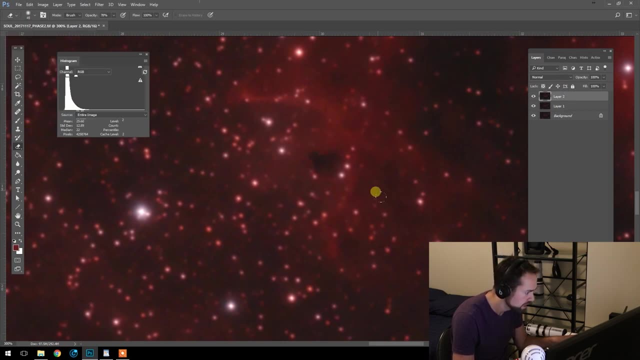 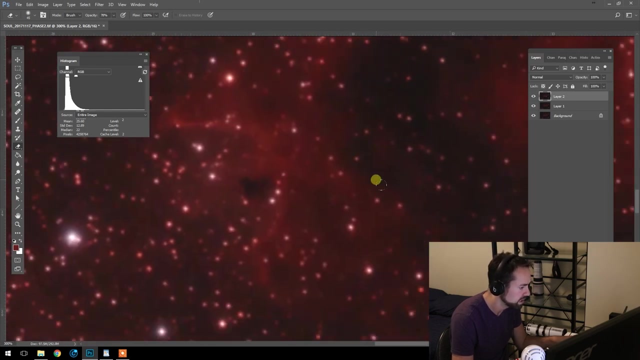 our new soft layer when I take it away it's there. so any selective areas that I want to smooth out? I would simply use the eraser brush and remove this top sharp layer, and I meant this can get really time-consuming, but if you really want that beautiful image, you'll go through it, the whole thing, and soften up. 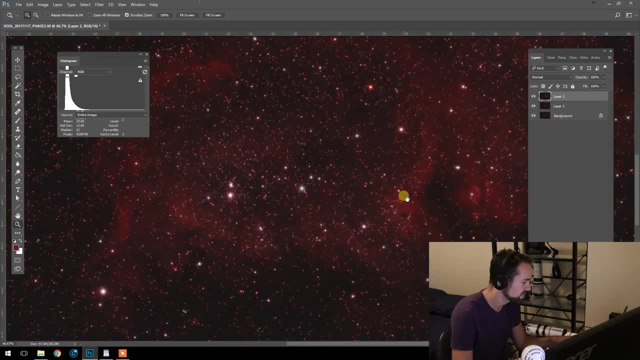 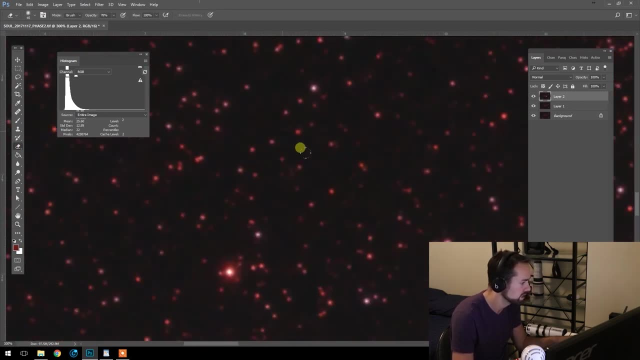 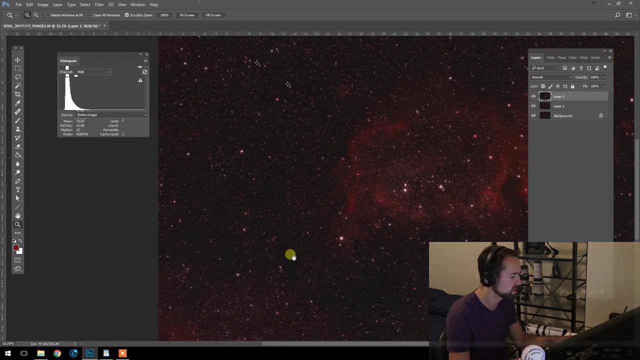 and smoothen those areas. so that's selective smoothing. and again, this you know it would be wise to do that here in the background sky you would pretty much want to take away. you could. you could smoothen most of this of the surrounding sky. the only areas you want to keep sharp are the nebulosity. so the final. 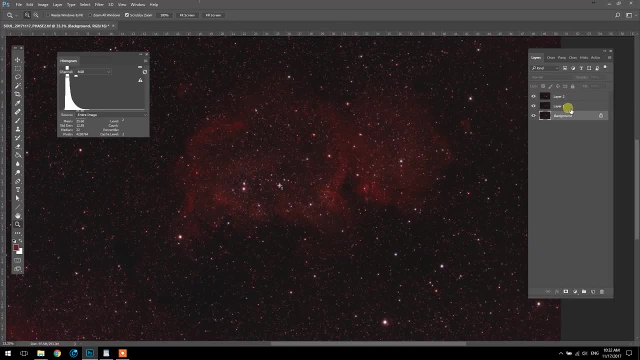 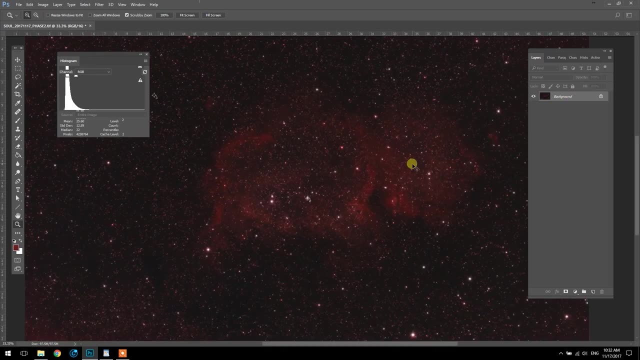 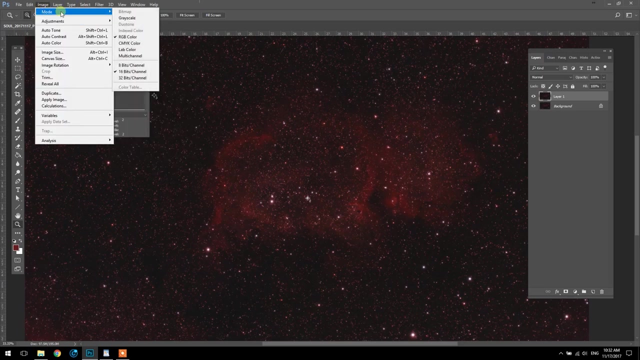 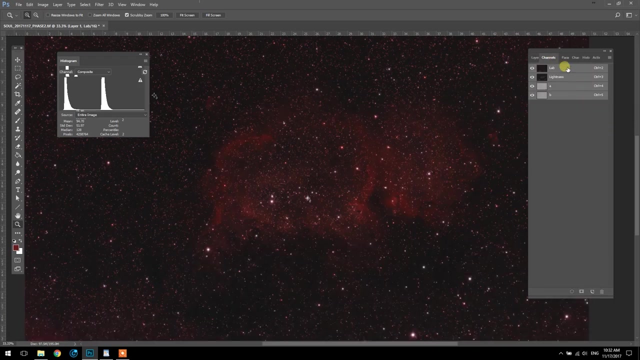 step of our image processing. here is: we'll be adding a luminance layer- very powerful technique. I'm gonna flatten everything, place my new layer on top and on this layer we're gonna go to mode lab color. don't flatten. and then, when we look at our channels here, 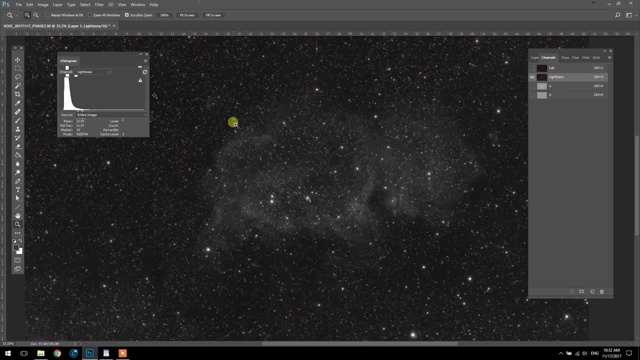 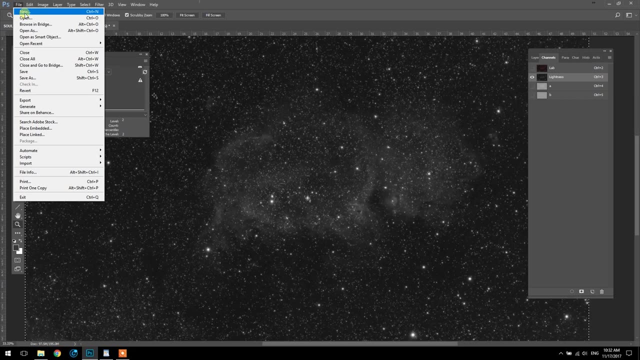 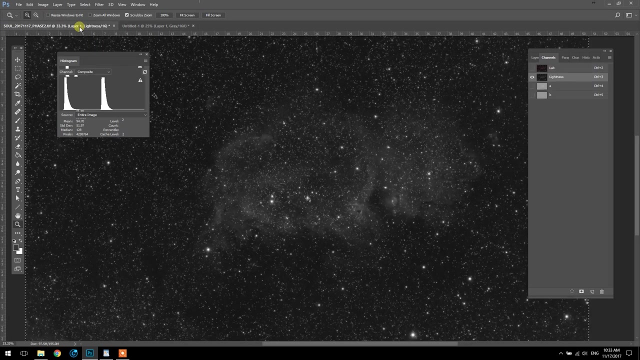 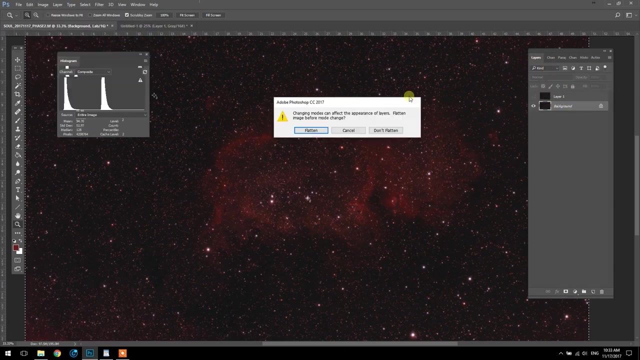 we want the lightness layer. so on this lightness layer I'm gonna ctrl a, cop, select all. ctrl C, copy, just to be safe. create a new document, paste, copy it again. sorry, my coffee maker is done. go back to our original image. here we can convert back the mode to RGB. we can flatten for these for this tutorial. 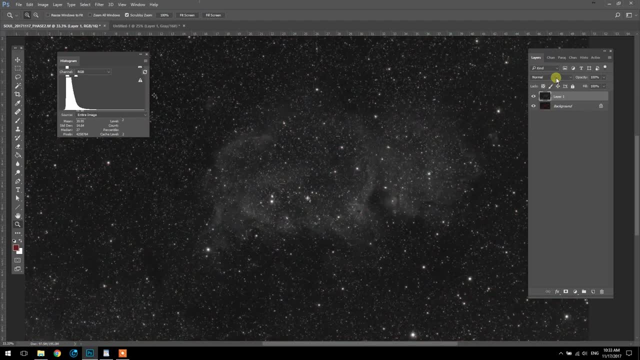 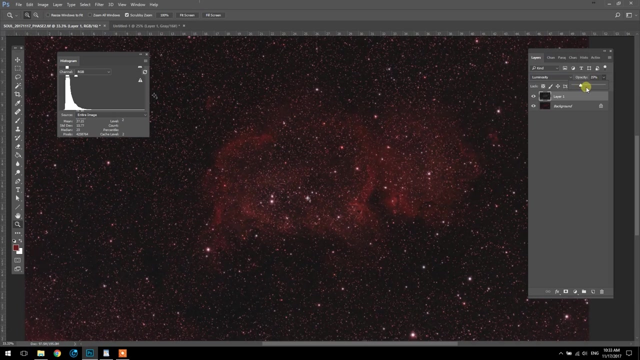 and then I'm gonna paste this lightness layer on top and what we're gonna do is change the blending mode to luminosity. so this is just brightening up the brightest areas of the image, which can be helpful for boosting contrast of your, your DSO. you won't want to use this at full opacity anywhere from you know, 50 to. 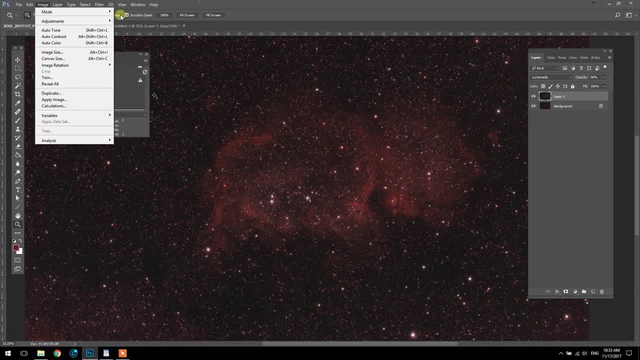 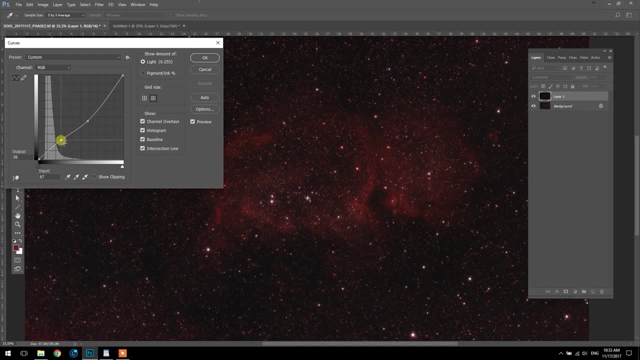 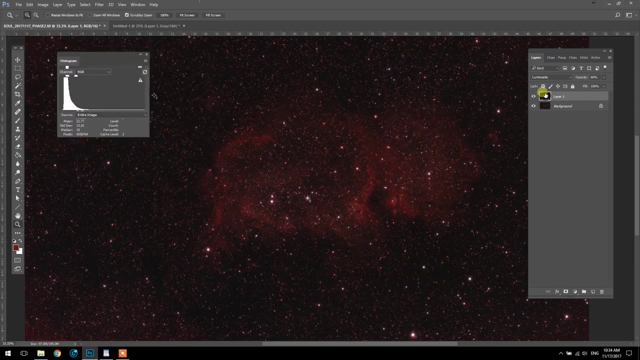 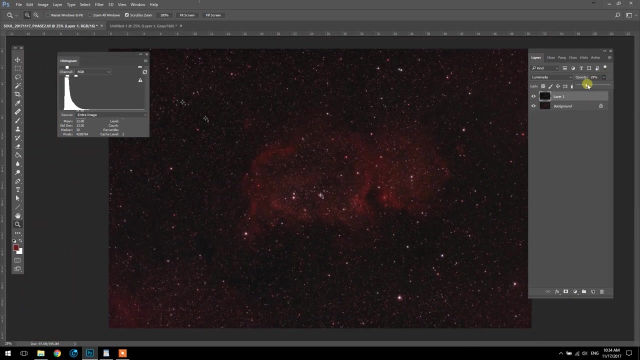 75 percent and then, when you've got it on there, you can make some curves adjustments. I recommend pulling the curve downwards so it's not so drastic, but you still get some of the extra boost you're looking for. here's the difference. you can see the difference in contrast that made. why don't we leave? 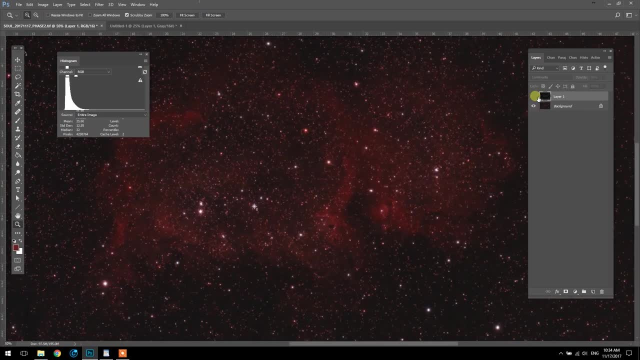 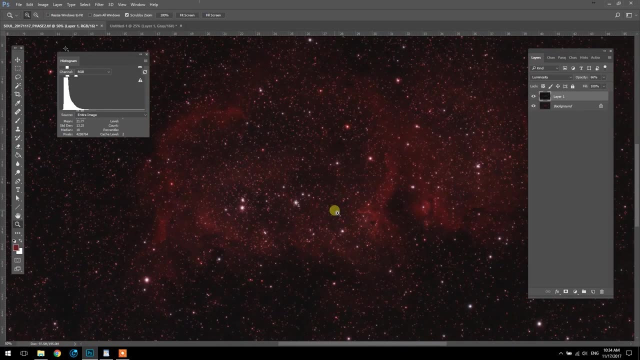 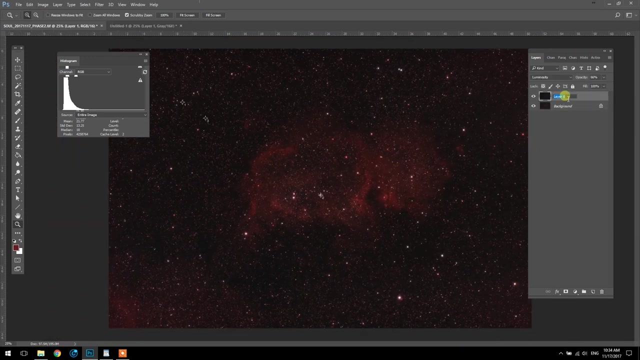 that about 66%. I'm rushing this stage. you could really spend a long time really mastering this. but we've darken the sky, we've boost the contrast, so that's our luminance layer on top. call that loom, move for luminance. and then at this: 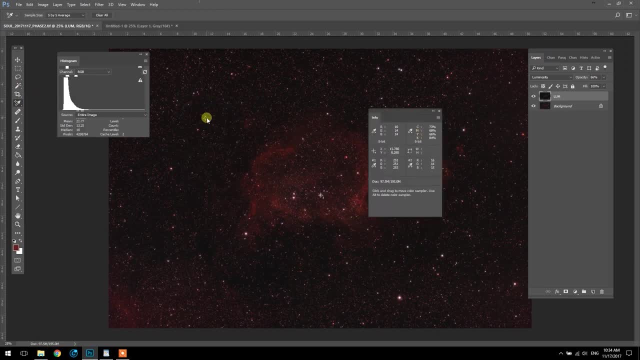 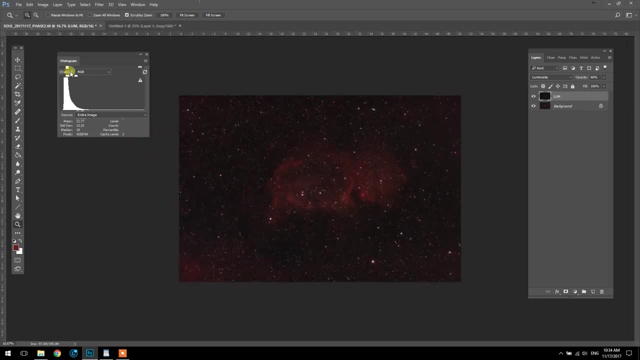 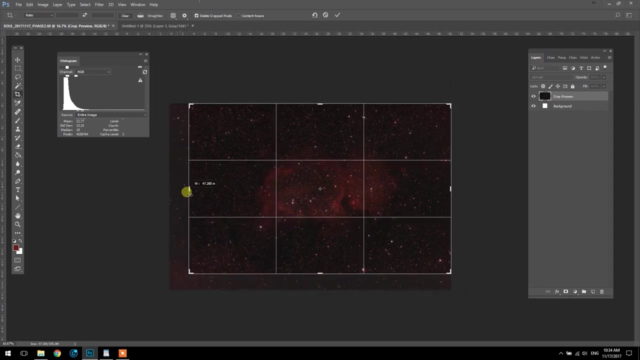 point. it would just be a matter of tweaking the image, finishing up just the way you like it, so we can take, finally, take these, these points off here, and for me I'd probably end up cropping this: say goodbye to that area of the heart nebula there. but I, I want to keep this wide field of view, and for this, 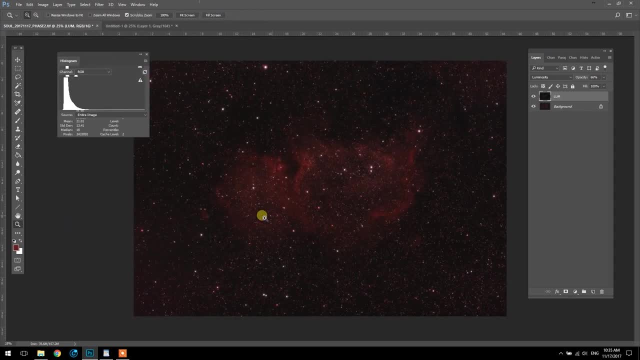 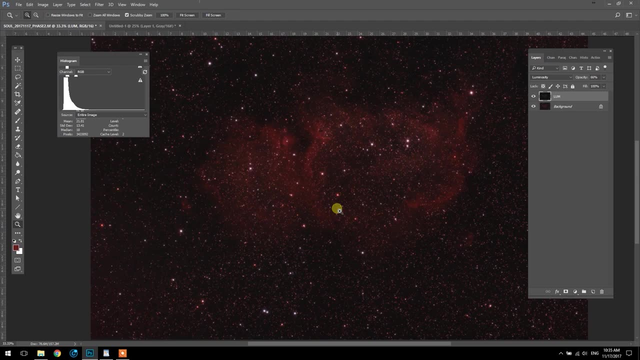 object. my final image. I have rotated it as well, kind of like the orientation here. so I hope you've enjoyed this tutorial and you've walked along the course with deep sky astrophotography image processing. there are so many ways to go about it and a lot of it has to do with your personal tastes, but at least. 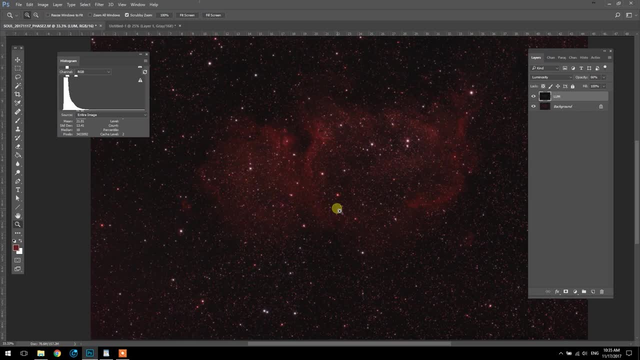 following these steps that I've shown you here, I think it's a good starting point for you to have some fun with not only this image but your own, so I really appreciate you sticking around for the whole tutorial. I hope you enjoyed it and I hope I didn't drive you too crazy with some of my steps, if you disagreed. 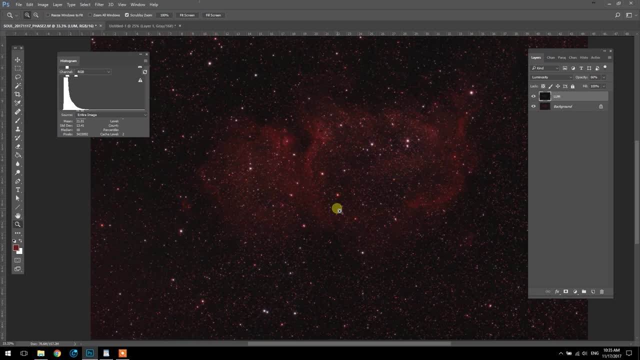 with the, the direction I was taking, but that's half the fun. so I'm gonna finish up this image. I'll share my final result at the end and, yeah, like I said, just have fun with it and and continue with this amazing hobby, and I hope this was useful. 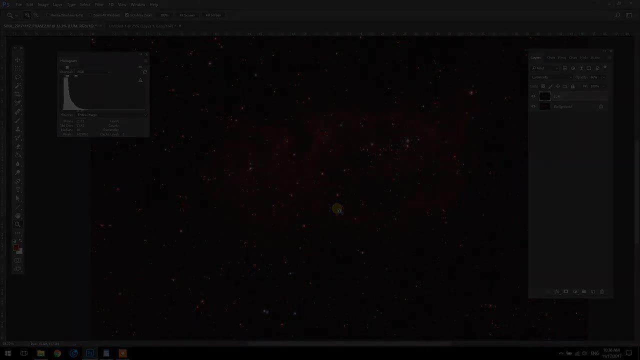 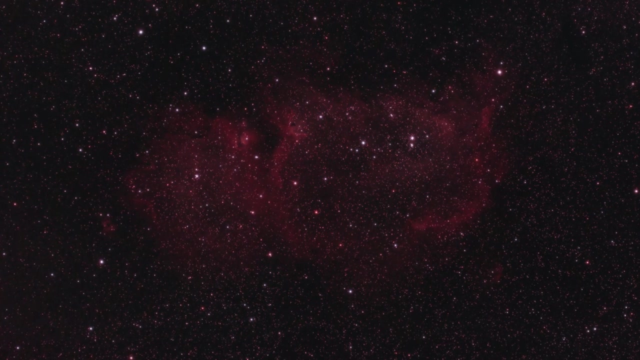 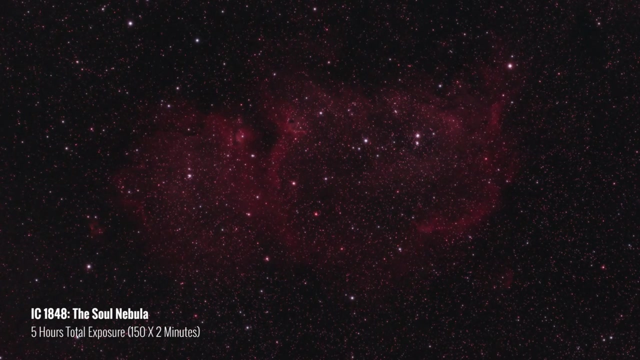 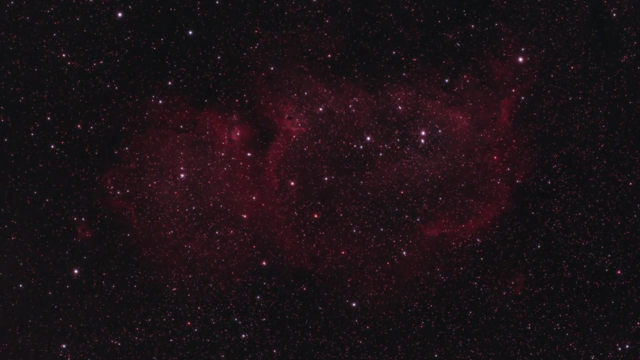 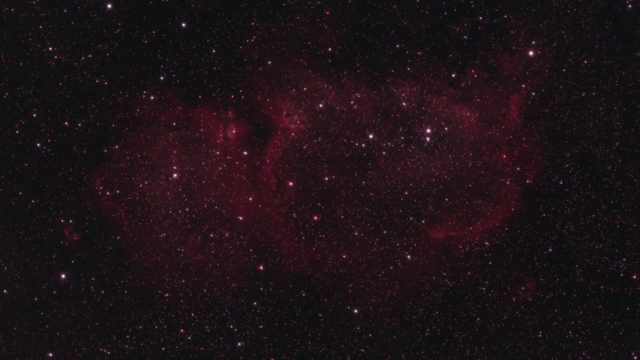 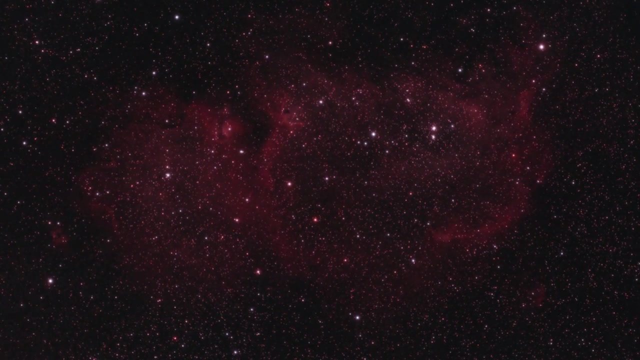 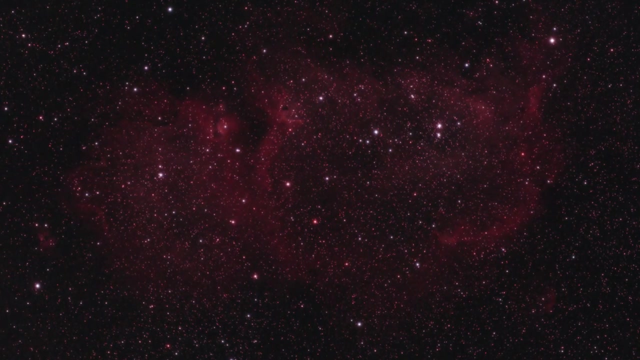 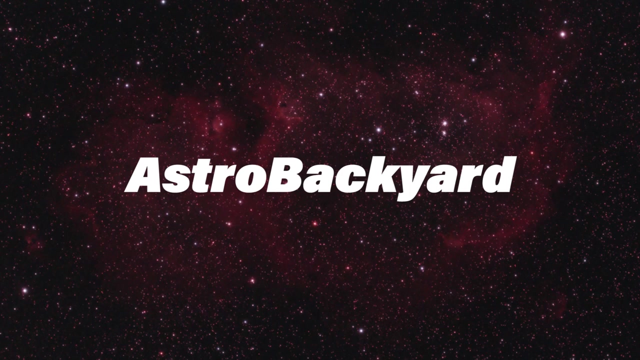 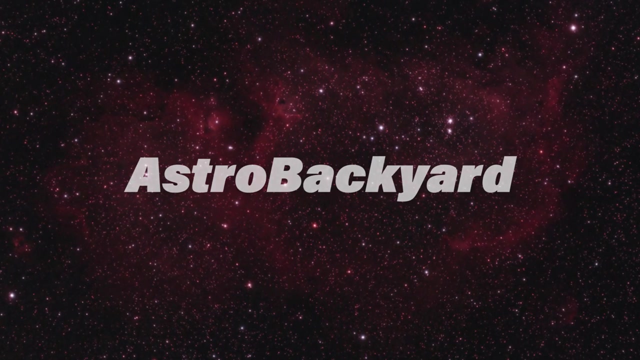 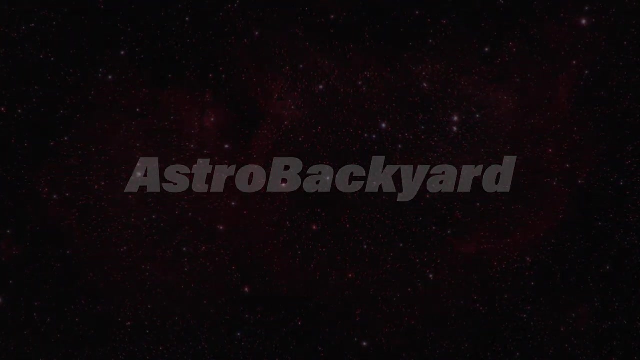